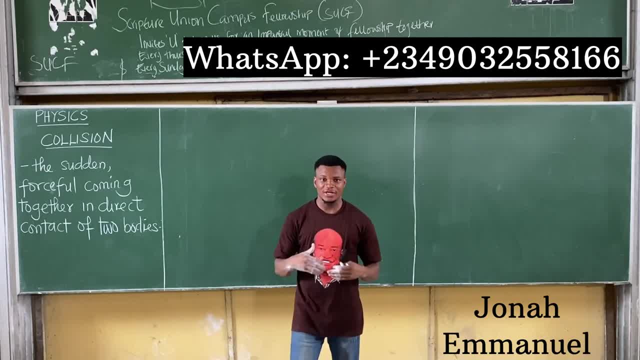 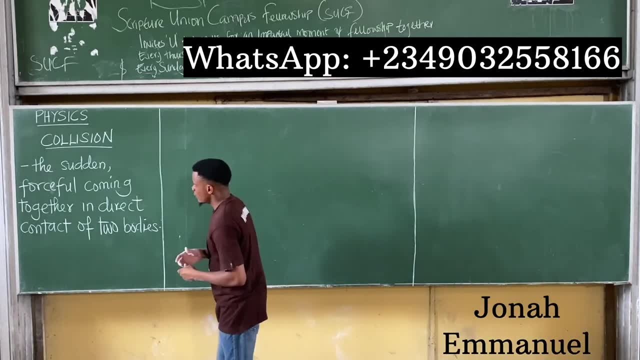 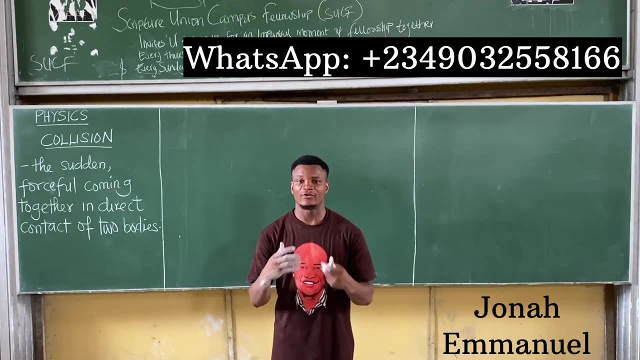 two bodies forcefully come in contact, suddenly and forcefully. That's how we define the term collision. alright, When it comes to collision. here, before we dive deep into collision, there are two sets of equations that are very fundamental or important in a discussion of. 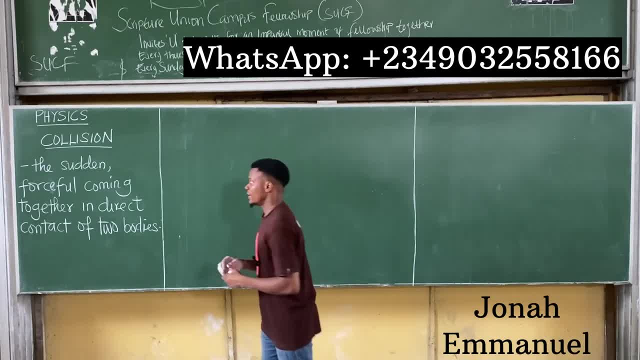 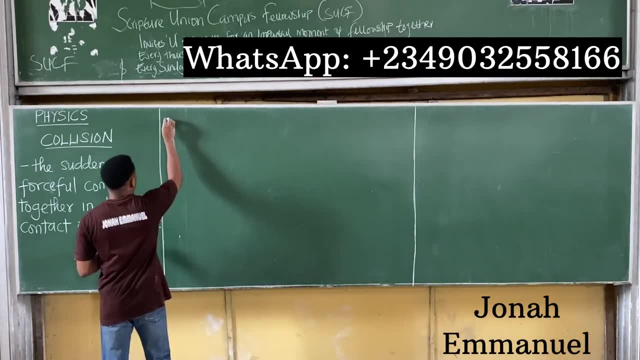 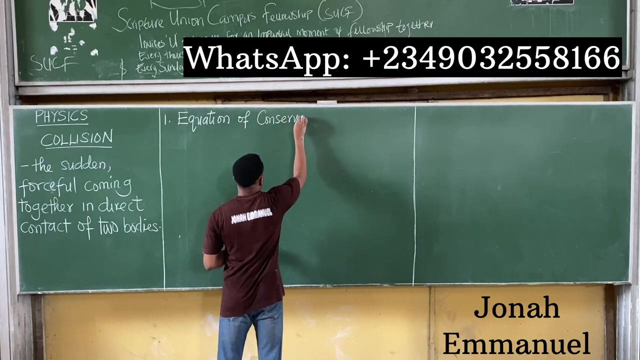 the concept of collision in physics. alright, Both equations are actually equations of conservation. The first equation there is called the equation of okay, The first one is called the equation of conservation. Conservation, the equation of conservation of momentum, or linear momentum if you want. 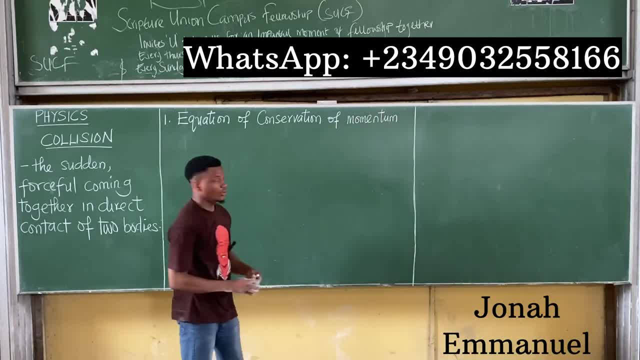 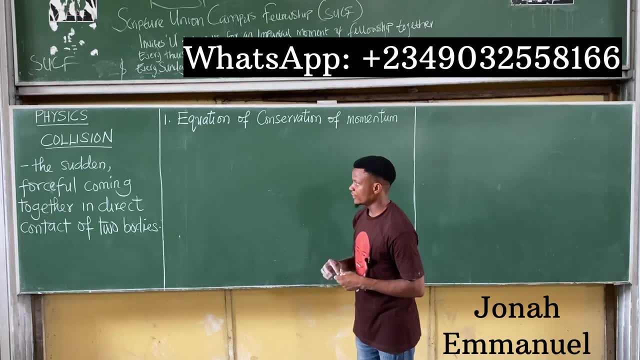 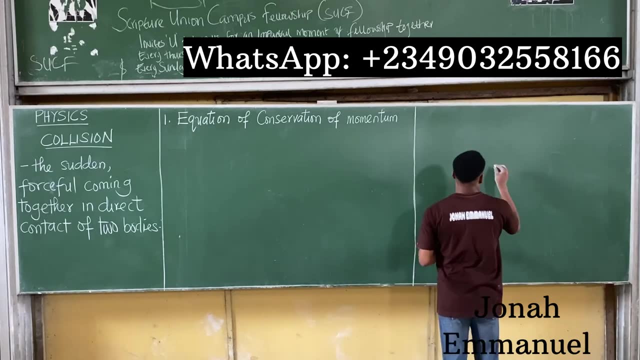 to okay. So the equation of conservation of linear momentum is the first very important equation in the discussion of the idea of collision. Before we look at this equation here, let's look at something, Let's consider something here. So consider that we have two bodies, two bodies. Let me 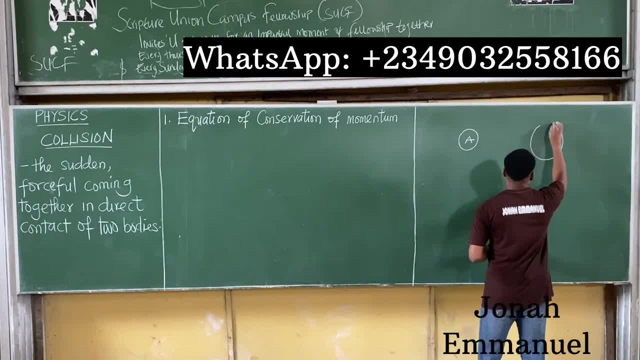 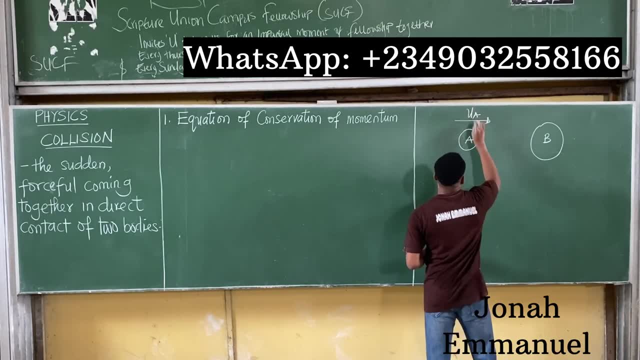 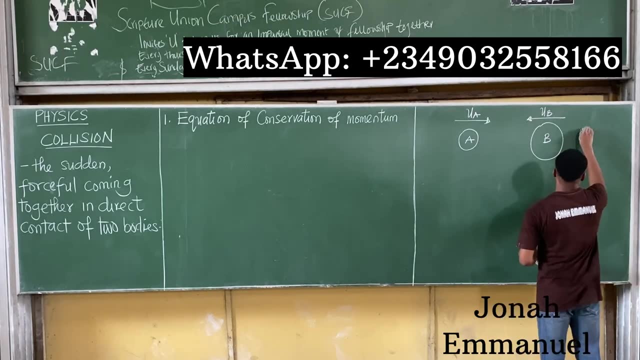 call this body A, Let me call this body B. So body A is moving with an initial velocity of, let's say, UA, and body B moves with an initial velocity of, let's say, UB. alright, This case is before they collide, or we can call it before collision. 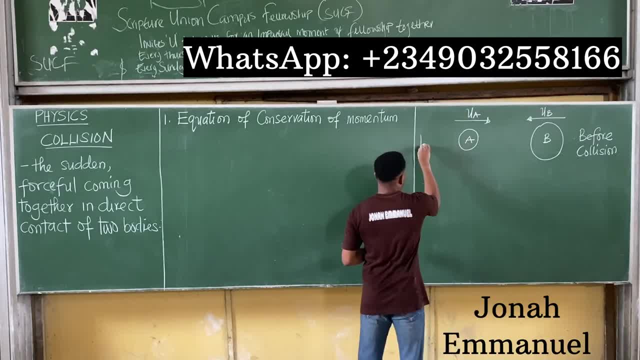 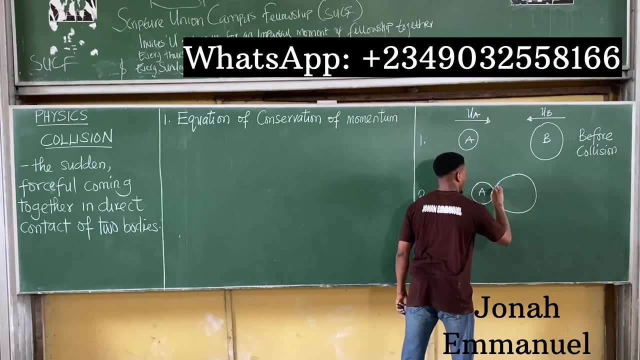 Alright, That's the first one there, So this is case A, or the first case, case 2.. Let's say they collide. Let's say they collide So during collision. I have something that looks like this: So body A collides with body B like this, such that they collide this way and 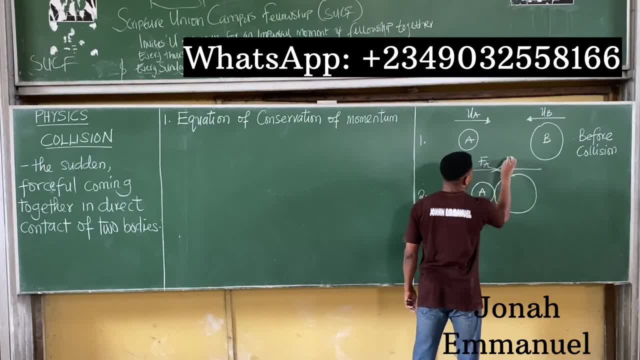 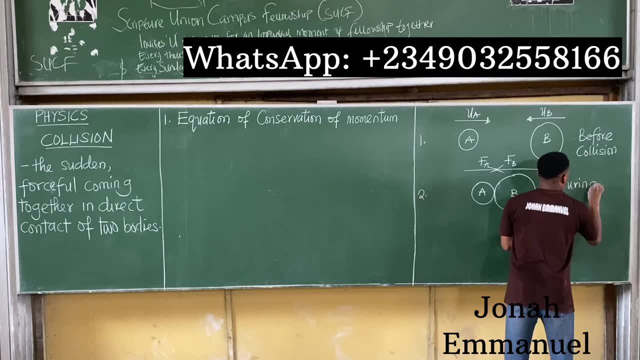 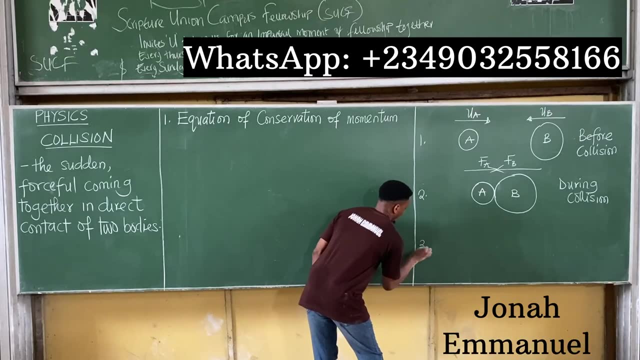 hit against themselves with a particular force here. alright, This is during collision, This is during collision, And then the third one there. finally, you now have a third case where they both move in perhaps the same direction, or different direction, as the case may be. 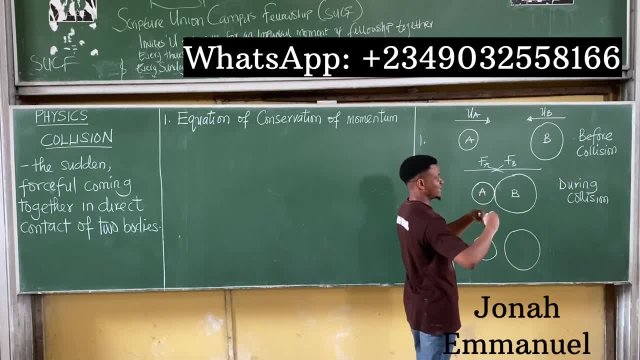 And I have that. Let's say they both hit against themselves and let's say, move in different direction per se, or let's assume that this is just an assumption that they move in this direction, I'll call this V-A and this direction here. I'll call this V-B. Okay, This is after. 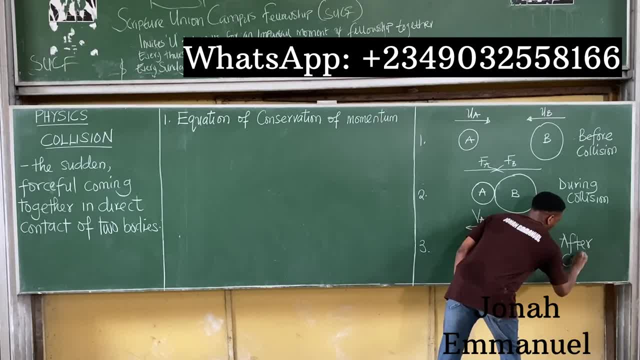 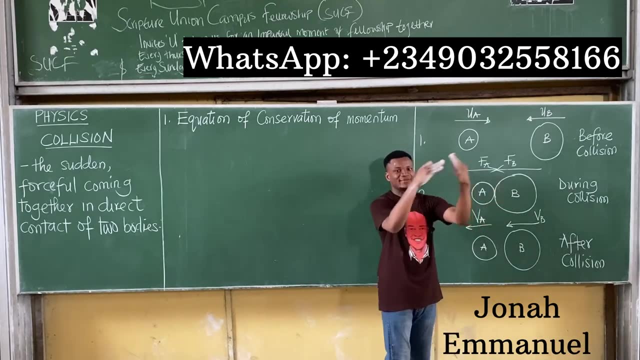 collision Alright. So consider this: I have two bodies Faces. first they suddenly or forcefully hit against themselves and they come together in direct contact, And that's what we have here as collision right. So they hit against themselves and then, after collision, let's say they move in. 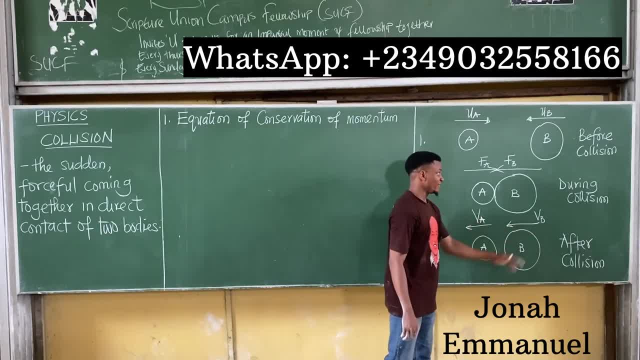 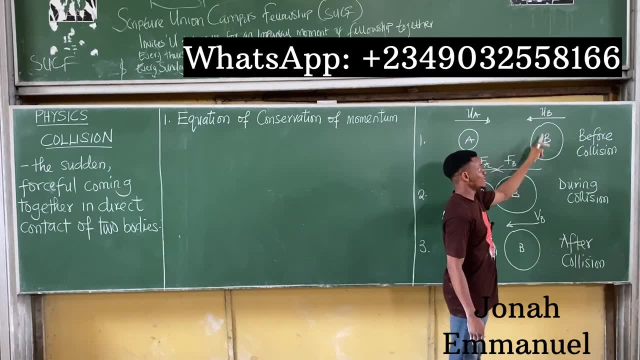 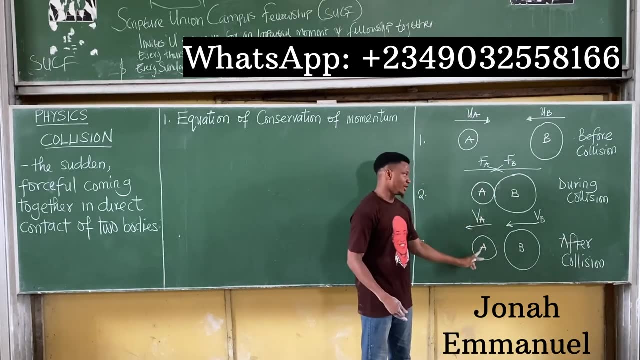 move with a different velocity: VA, BB, Alright. so UA is the initial velocity of body A before collision, UB is the initial velocity of body B before collision, VA is the final velocity of body A after collision And BB is the final velocity of body B after collision. 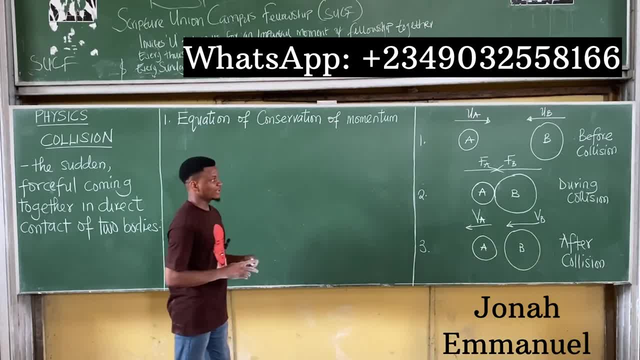 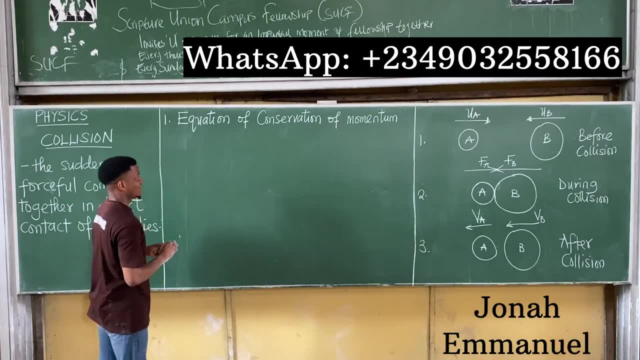 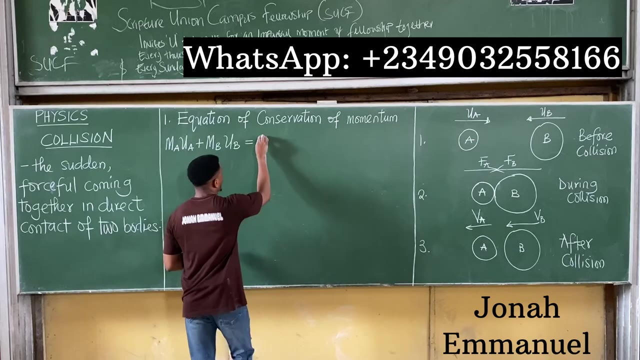 From this here there are two important conservation equations that we can get here. The first one is called the equation of conservation of momentum, And we've gotten this in our previous class. We said this is MA or M1, if you want to. UA plus MB. UV is equal to MA- VA. 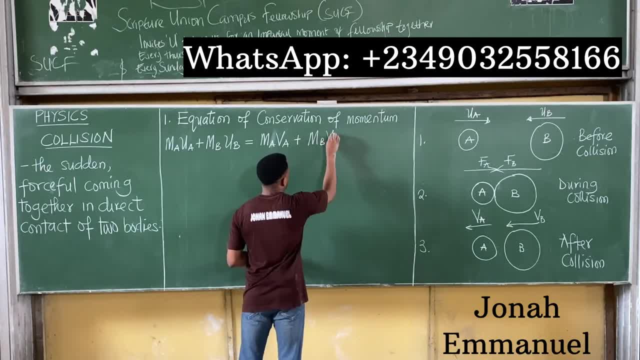 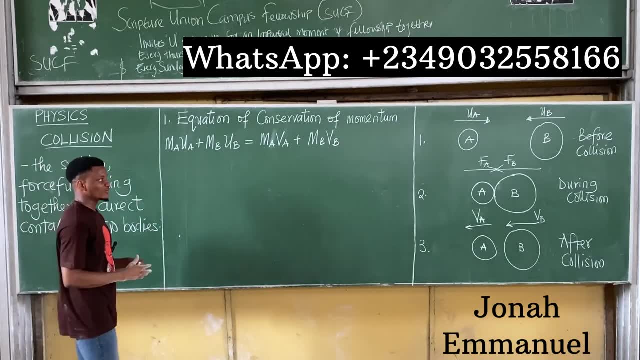 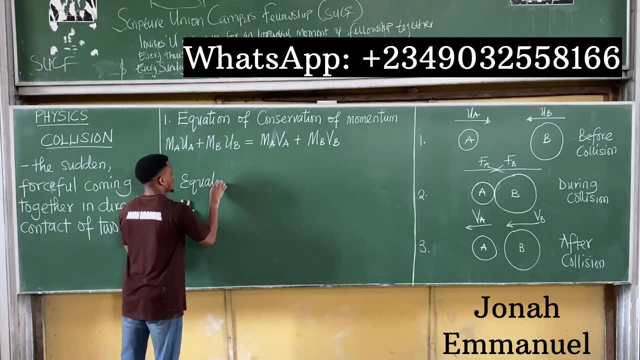 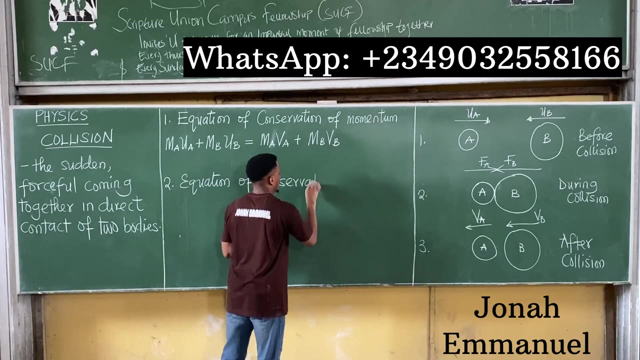 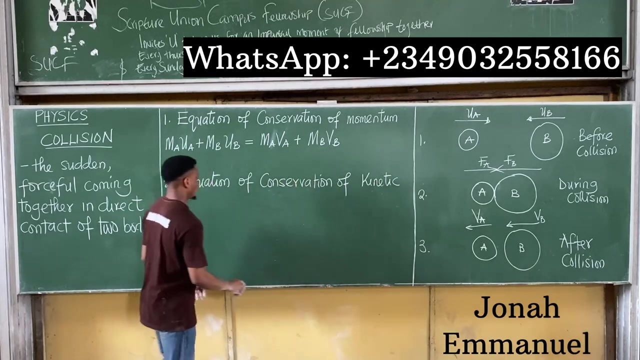 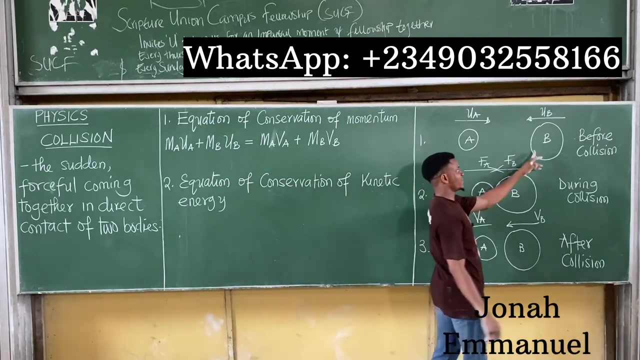 Plus MB, VB, Alright. so this is the first law, or the first equation of conservation for linear momentum or momentum. The second one is the equation of conservation of kinetic energy, Very important, Important of kinetic energy. So, since these two bodies are moving at a velocity, they will have kinetic energy because they are in motion. 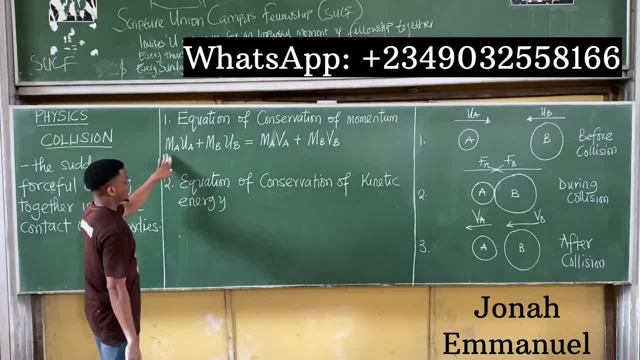 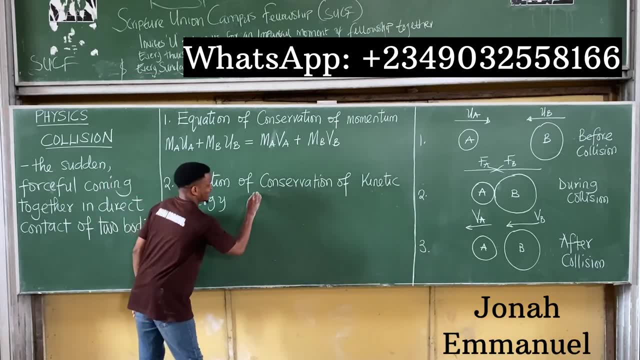 Alright. so how do you write this equation for kinetic energy? It will be the same thing as this, just that it will take the form of kinetic energy. What is the form of kinetic energy? Remember that we said: kinetic energy is equal to half multiplied by the mass of the body. 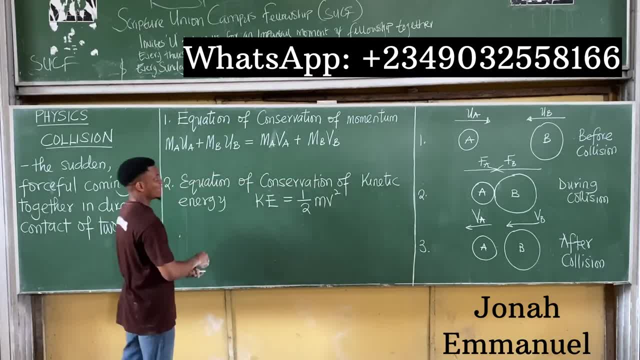 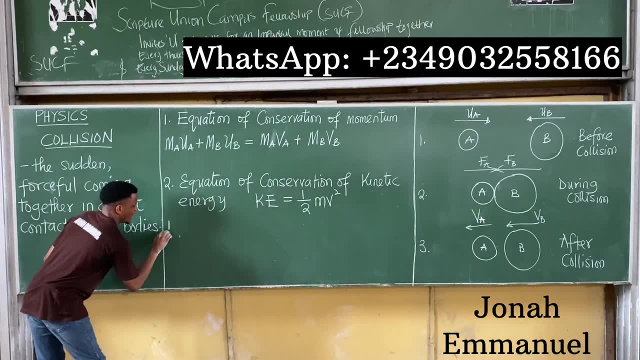 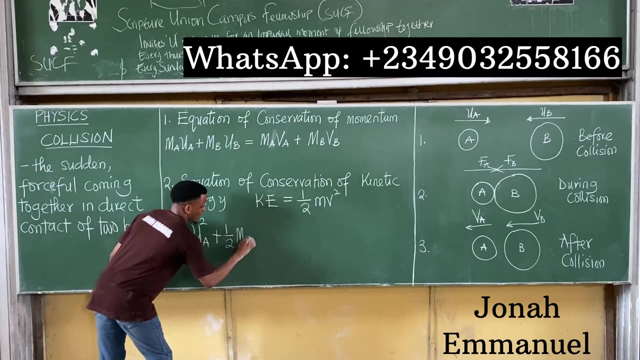 Multiplied by the square of its velocity. So I'll just attach half to each of them and I'll square each of the velocity, So this one becomes half into ME. yeah, UA square, the velocity squared, plus attach half again. half into MB, UV squared. 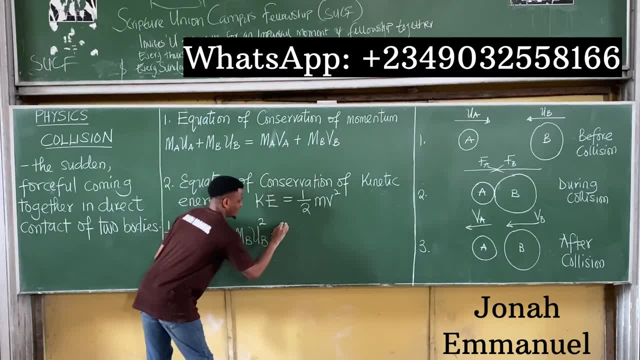 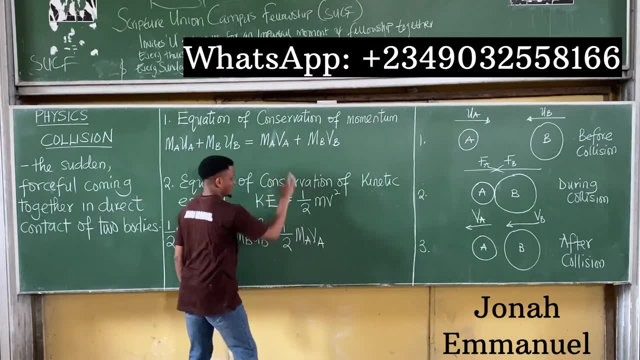 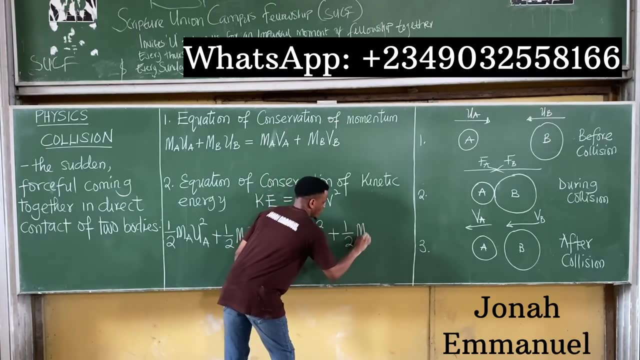 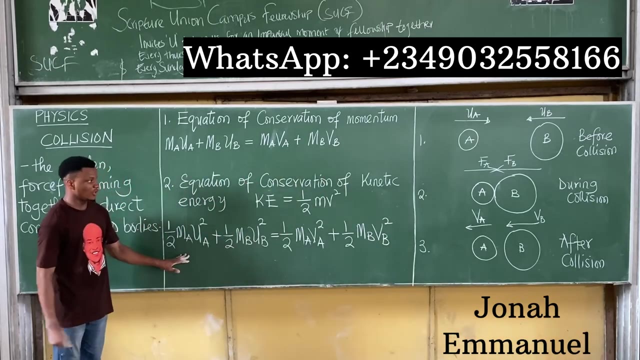 is equal, Okay, Okay, equal to. from here: attach half, half M A, V, A square, this man squared plus. so this one here becomes half into M B, V, B squared. Alright, so this becomes the equation of the. 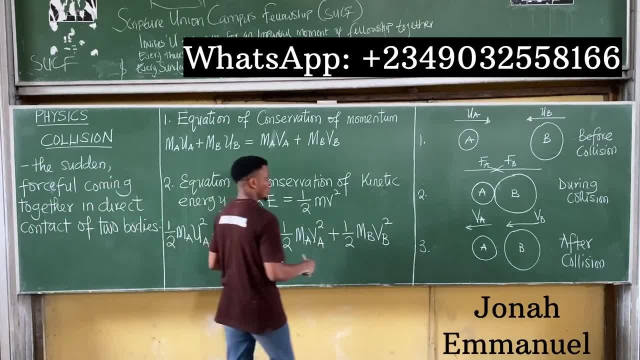 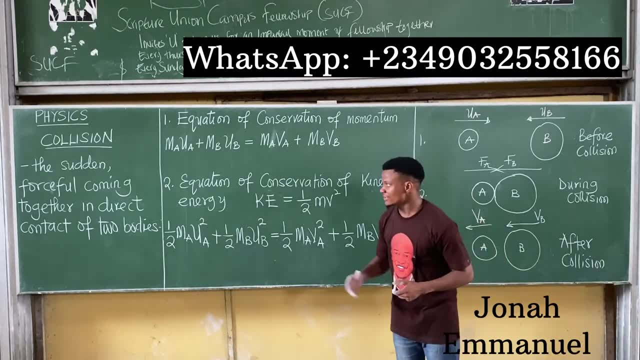 conservation of kinetic energy. Alright, so, having considered these two cases, so having considered these two cases, we'll now look at the types of collision. Basically, we have two types of collision. The first one is called the elastic collision, and then the second. 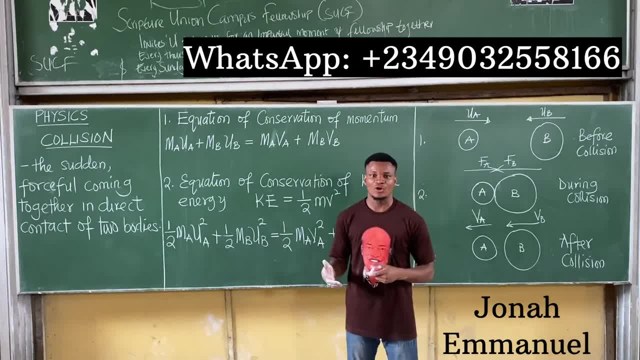 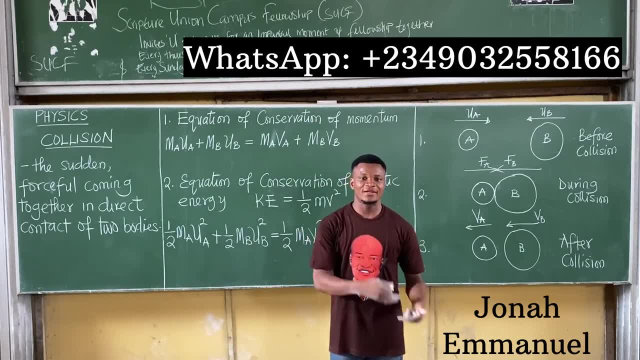 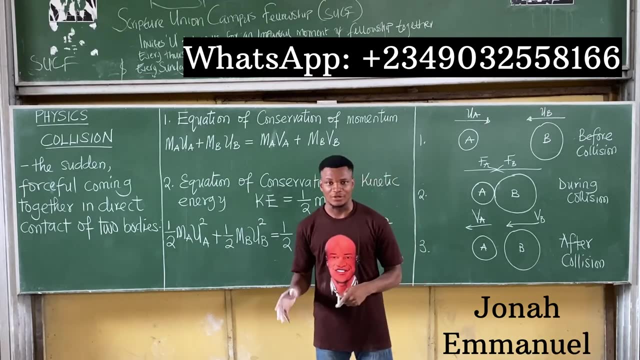 one is called the inelastic collision. But aside these two, we also have other types of collision. Example: the perfectly elastic collision. we also have the perfectly inelastic collision. alright, And what have you So look at? let's look at the two basic types of collision. which is elastic? 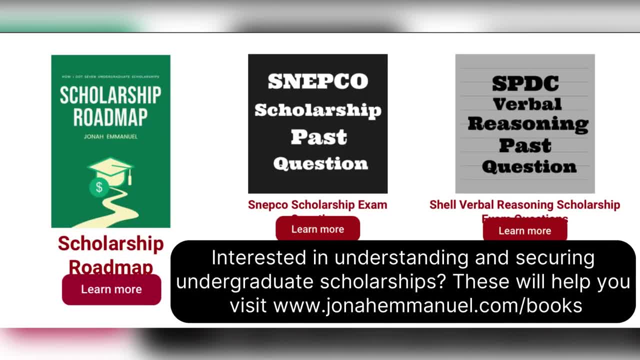 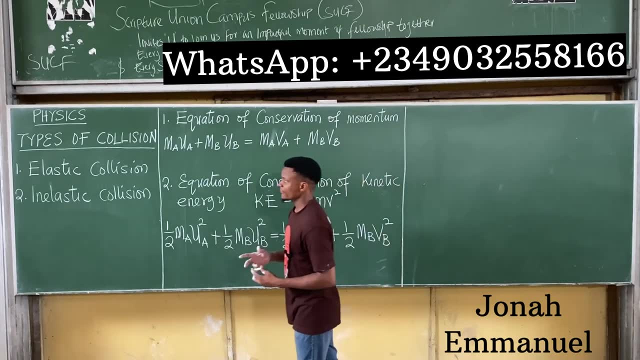 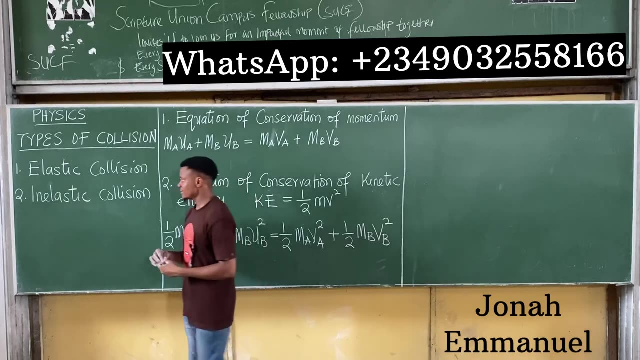 collision and inelastic collision. Alright, let's discuss the types of collision Now. basically, there are two types of collision: the elastic collision and the inelastic collision. Now, how do we differentiate? How do we differentiate two of them? Let's start with the first one there. Let's start. 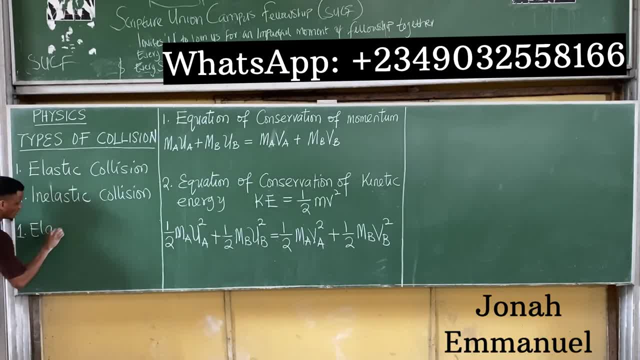 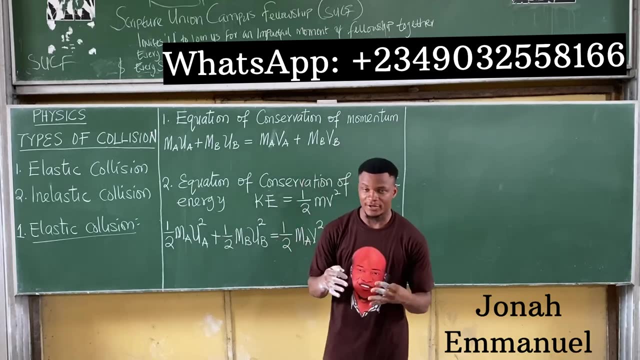 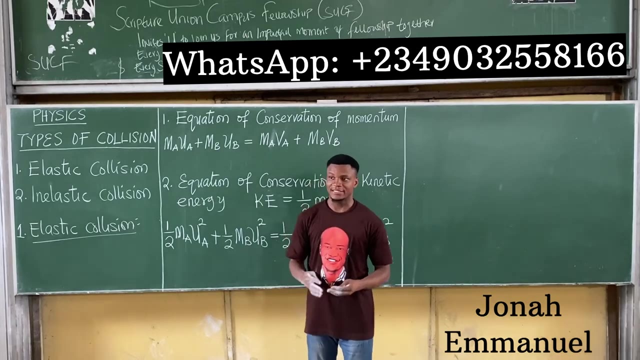 with number one, elastic collision. Let's start with elastic collision. Alright. Now here's something to note. please For elastic collision after the collision process. alright, the two bodies undergoing the collision move at different velocities after collision. alright, That's. 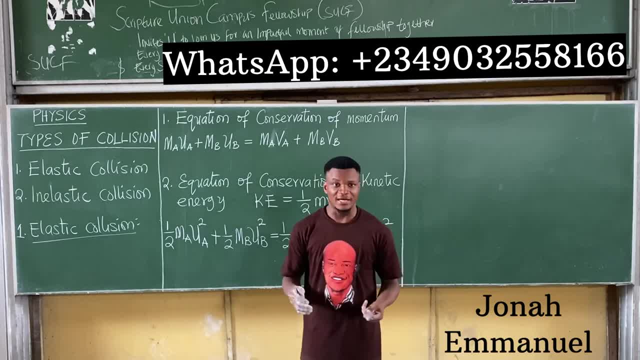 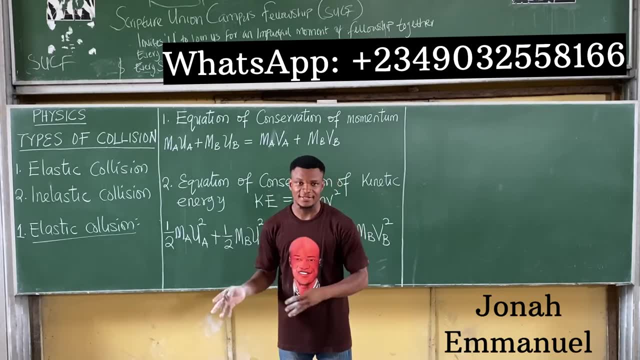 like the key idea about elastic collision. So for elastic collision there we say, when two bodies collide, after the collision process they move at different velocities, alright, after collision, And that's kind of collision is called elastic collision. Now remember that we said we have two important equations. 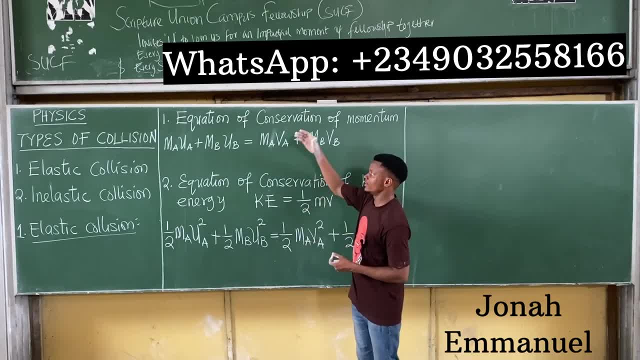 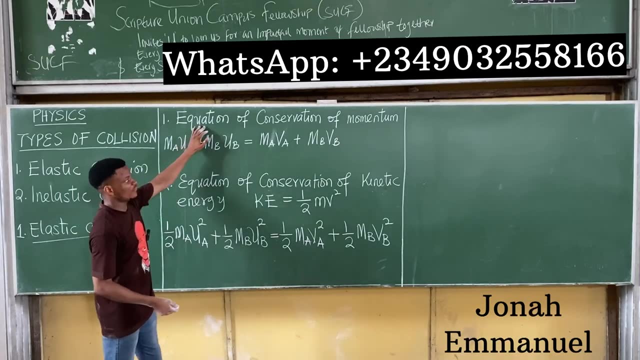 for collision, which were the equation of conservation of momentum and the equation of conservation of kinetic energy Under elastic collision. Since the body moves with different velocities, we have that under elastic collision, the equation of conservation of momentum remains the same, alright. 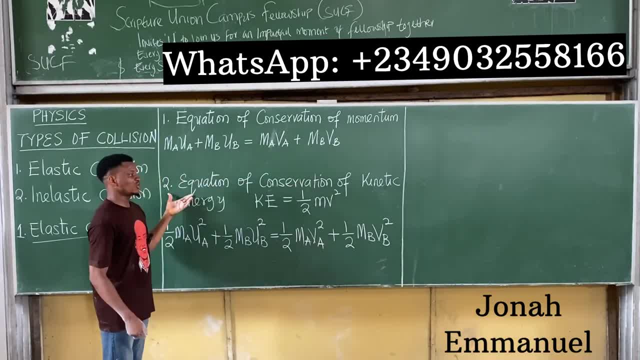 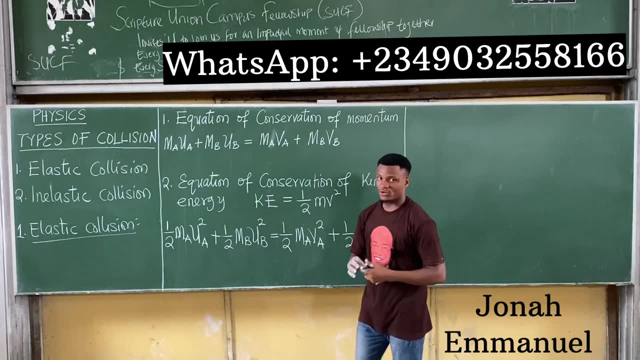 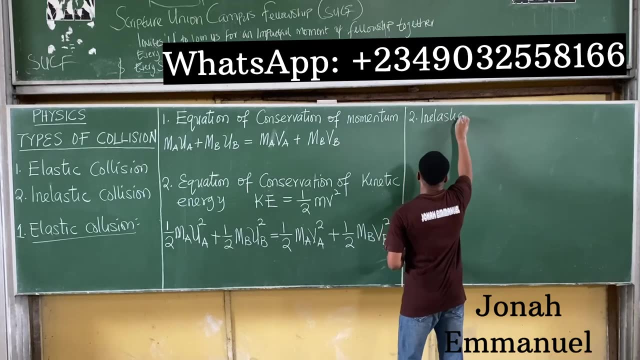 You have different velocities. Also, the equation of conservation of kinetic energy also remains the same. So this same thing works for elastic collision. alright, Number two, let's look at the second one. They are called inelastic. Let's look at inelastic collision. 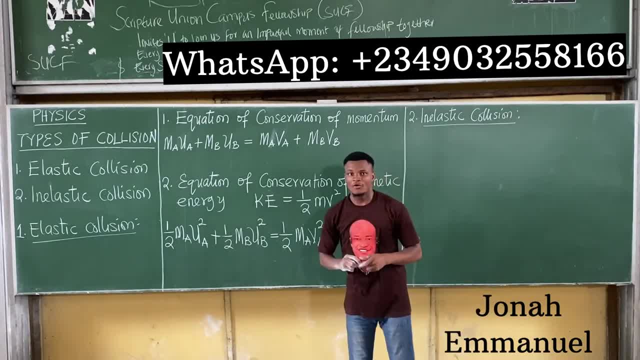 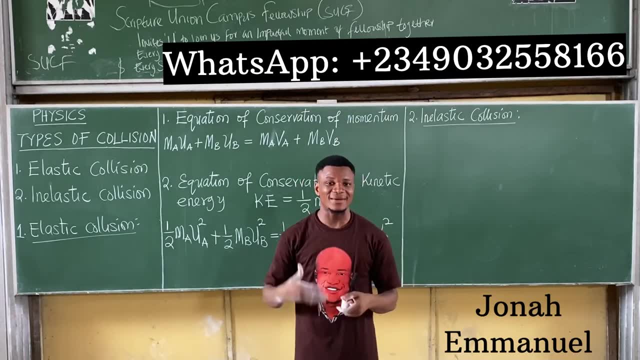 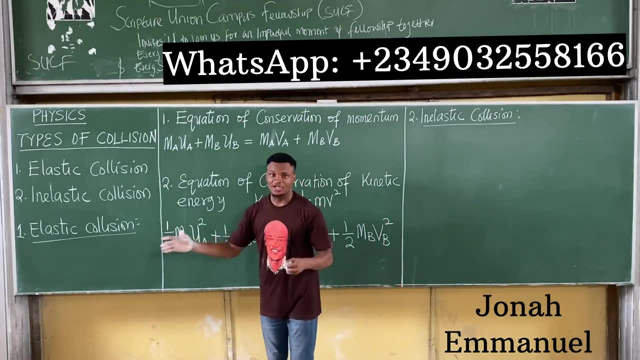 Alright. so what is inelastic collision For? inelastic collision, after the collision process, the bodies combine and move with the same velocity. alright, That's the key difference between elastic and inelastic. alright, After collision. for elastic, the bodies move with different velocities. 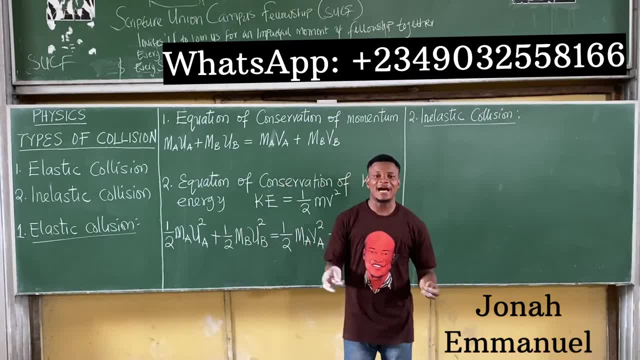 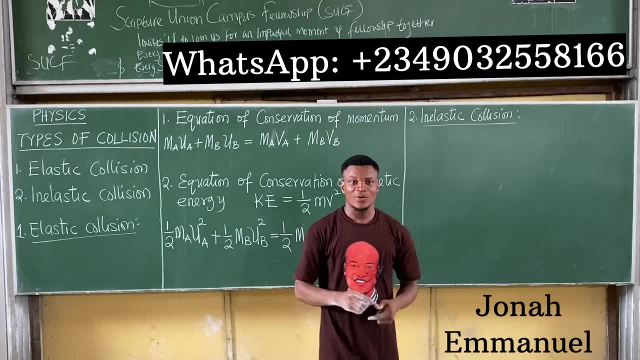 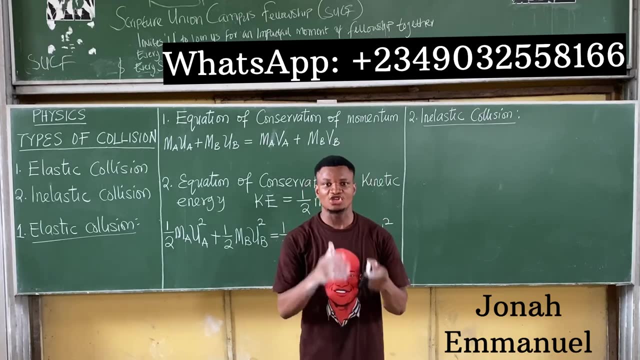 Why? for inelastic collision? the key idea is that after the collision process, the body moves with the same velocity After collision, After collision. So we are saying that for inelastic collision, the velocities of the body after collision is usually the same. alright, 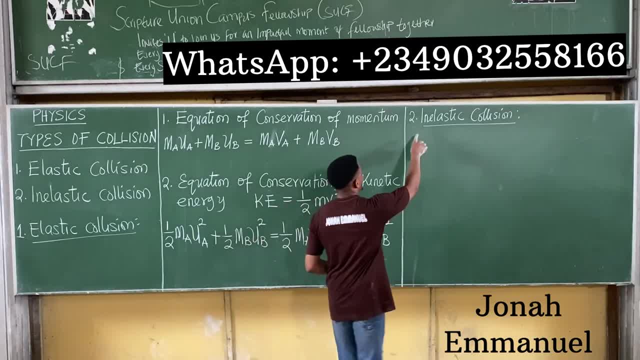 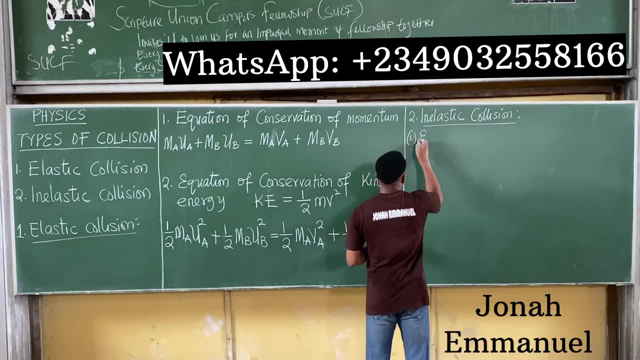 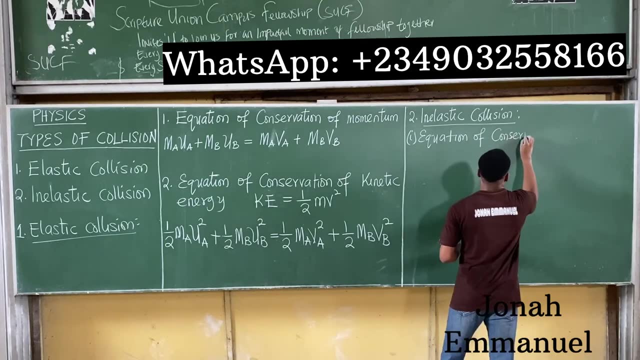 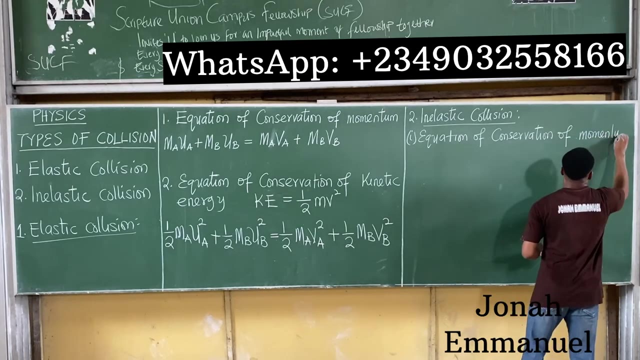 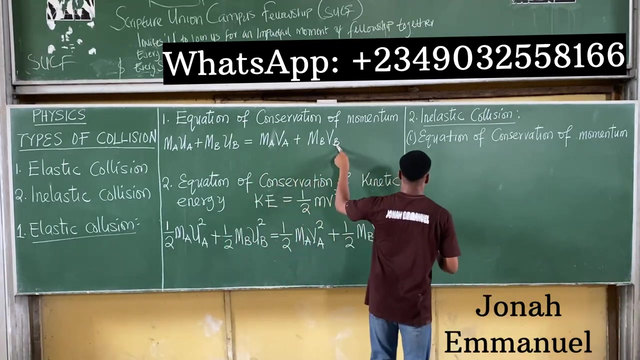 Now, if that's true, what do we have? We would have that for inelastic collision, the equation of conservation of momentum. So under this number one, the equation of conservation of momentum would be this: Now, here's the idea. We're saying that for inelastic, that VA is equal to VB. 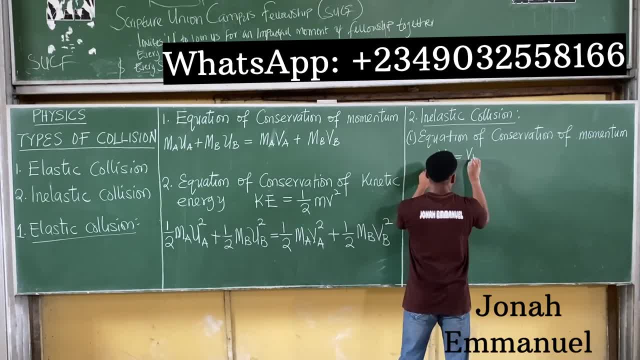 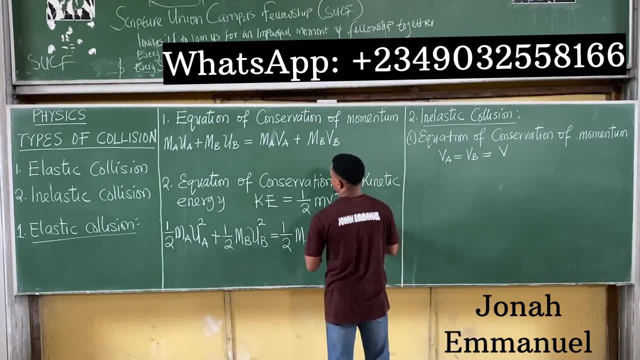 That means the final velocities is equal to VB and since they are equal, let's call them one thing and let's call them V. So if we call them V, we'll have something that looks like this: Don't forget, the initials are not the same. 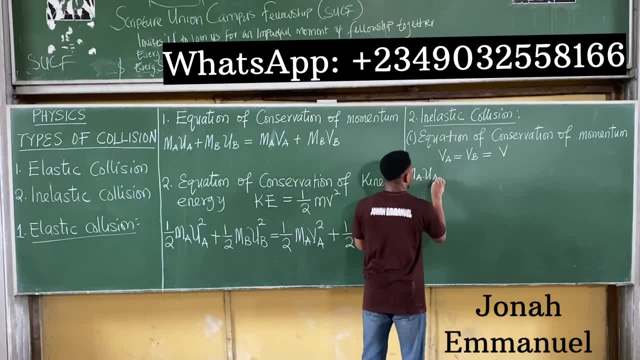 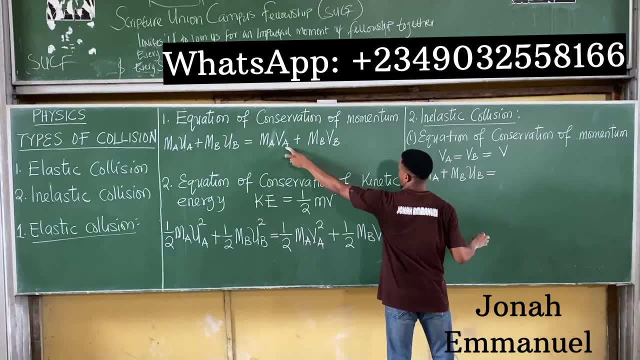 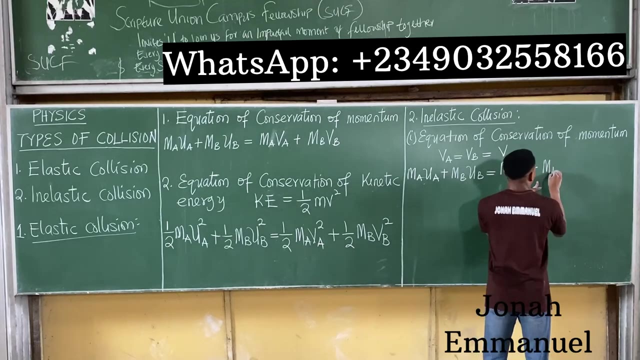 So I'll have something that looks like MAUA. MAUA plus MBUB is equal to MA MAVA, But VA is the same thing as VB and we chose to call it V. So into V plus MB. so I'm having MB- VB, alright. 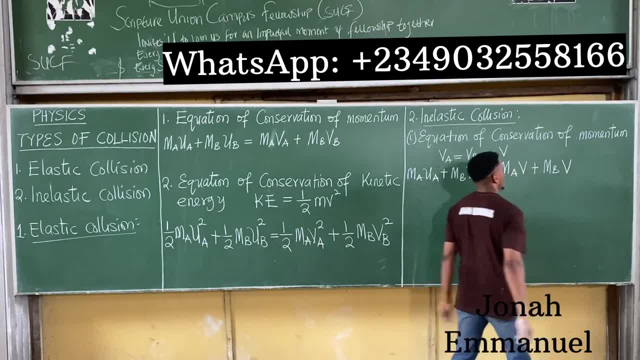 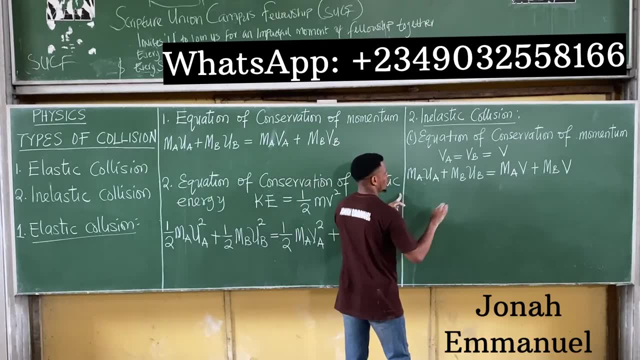 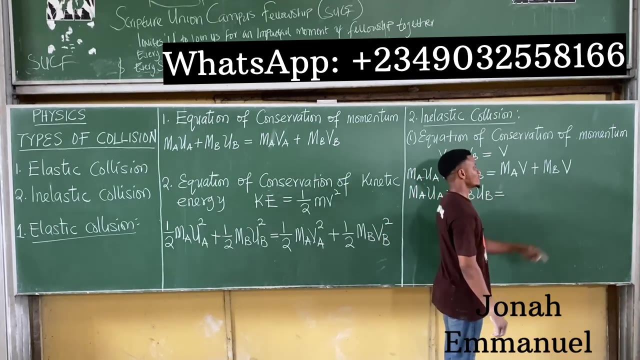 VB and VA are the same. We called it V, So I have this. Alright, so it would look like this. Now for inelastic collision. if I factorize, I will now have something of this nature. I'll have something that looks like: MAUA plus MBUB is equal to factorize the V out. 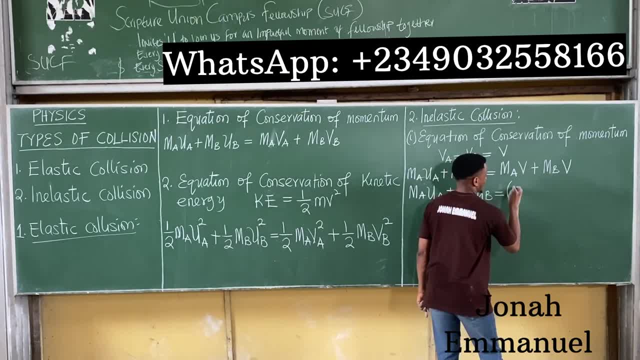 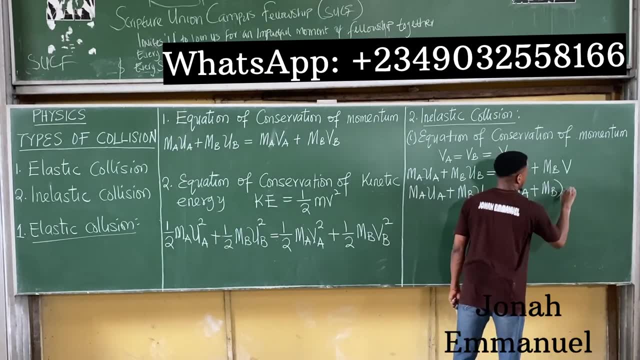 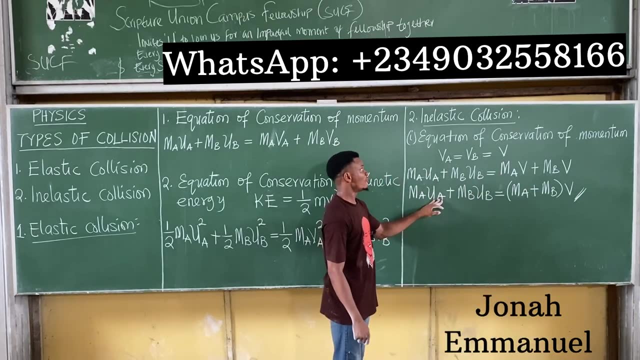 If I take out V- here you left it MA, so it becomes M, subscript A. plus, take out V- here you left it MB, So MB into V. This is the equation of conservation of momentum, or linear momentum for an inelastic collision. 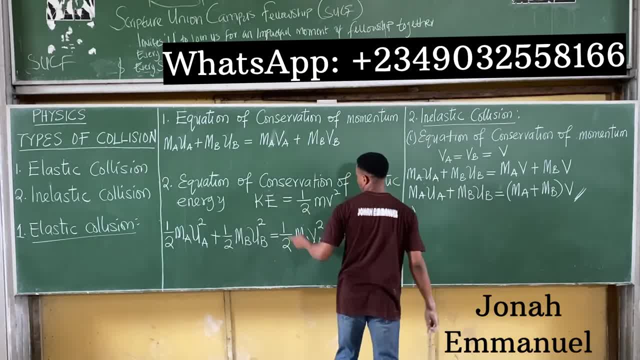 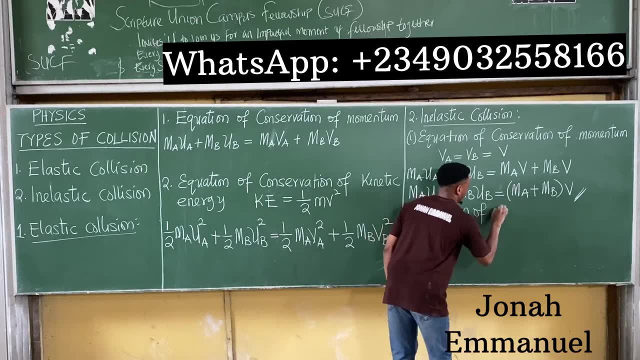 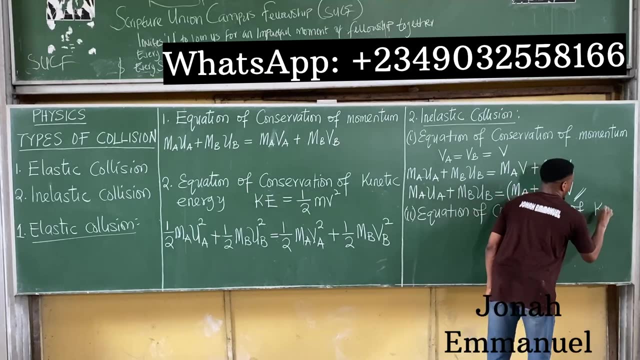 Alright, let's look at the second one there, which is the equation of conservation of kinetic energy. So equation of conservation of- Let me write this as KE- This KE here means kinetic energy- Just to save, Just to save space. 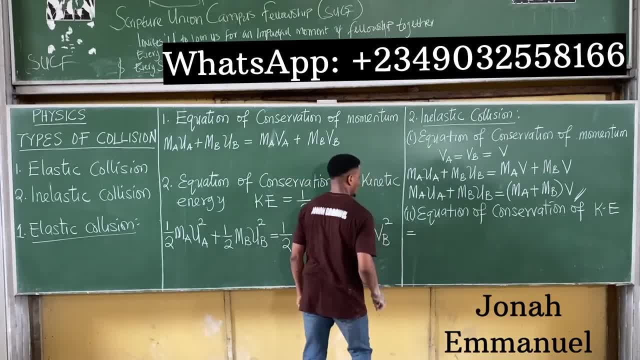 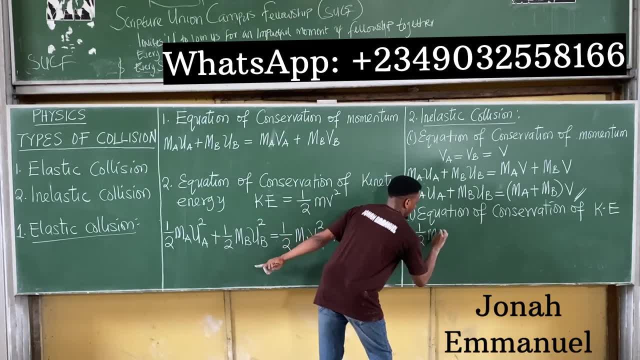 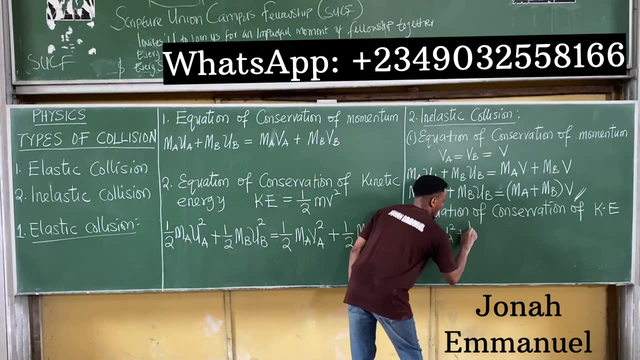 So what would that be? That would be equal to This, would be equal to half. I'm having half MA UA squared, So just this plus half MBUB squared, That's this. It's equal to half MA MA into VA squared. 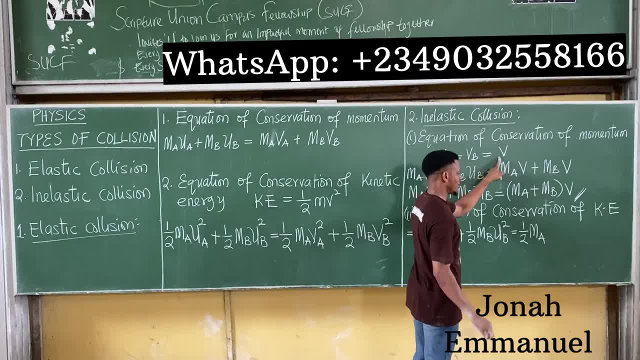 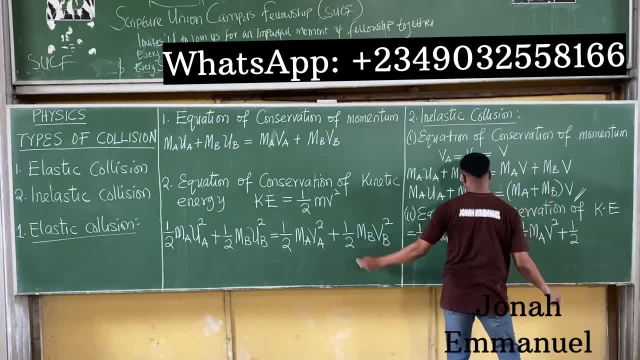 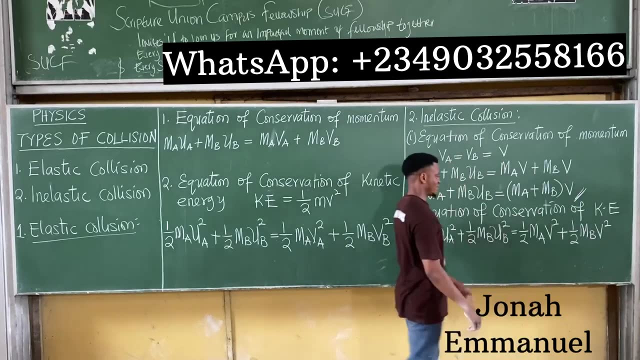 But VA is equal to VB and that's equal to V, since they are the same. So it becomes V squared plus half. that's this one here. into MBVB It's written as V, all squared. So I have this. 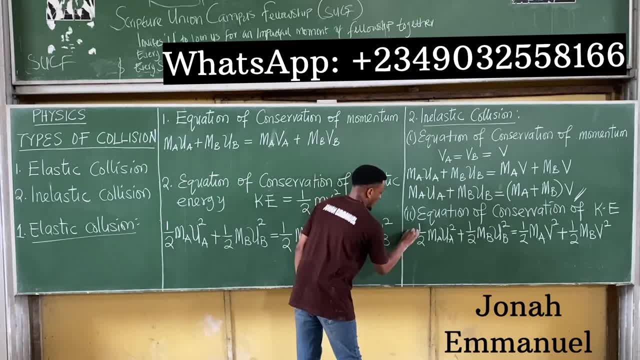 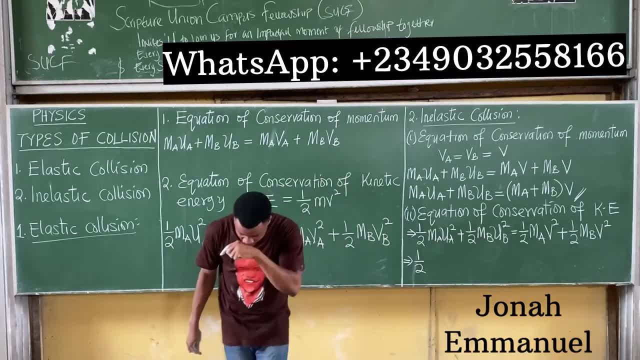 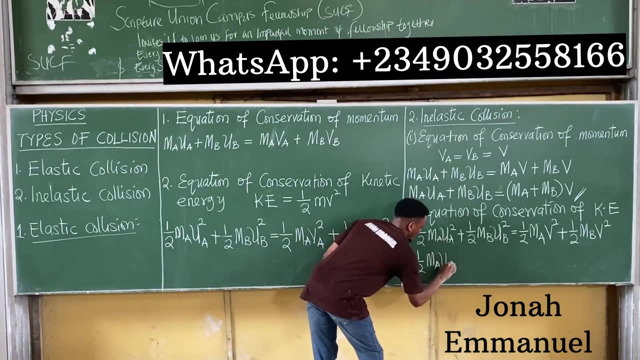 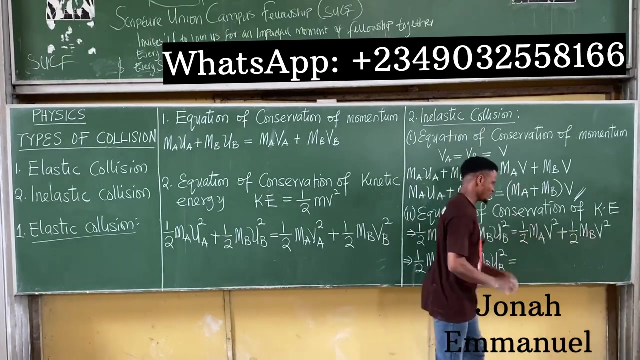 Also, we can still factorize this If we factorize. okay, If we factorize, we'd have something of this nature: Okay, That would be half. That would be half into m a? u a squared plus half into m b? u. b squared is equal to: I can see v squared. I can see v squared. 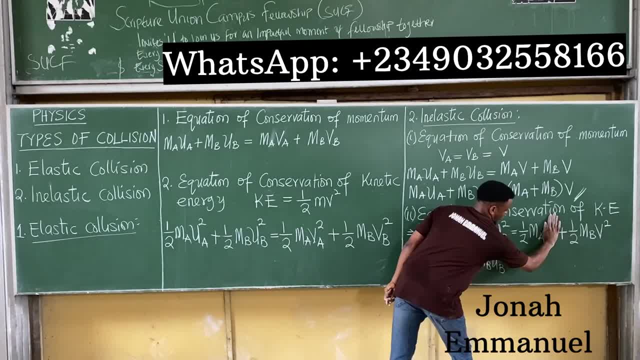 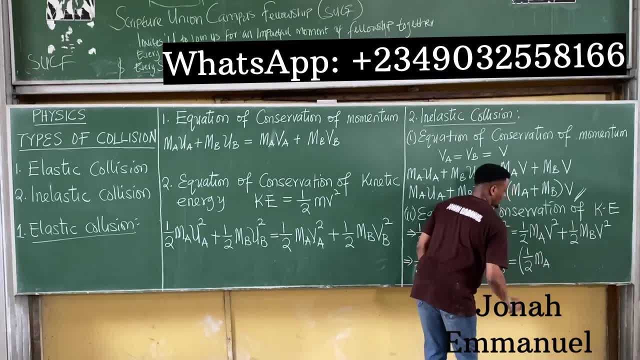 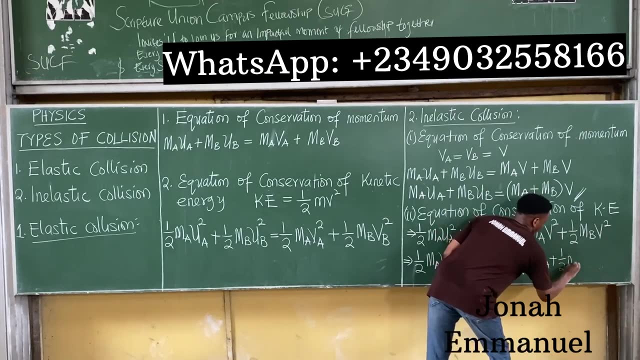 Take out v squared here, You're left with half m a. So half m a is left. That's equal to, in brackets, half m a plus. take out v squared here, you have half m b. That's half m b, Alright. So I'll be left with what there? V squared, So v squared. 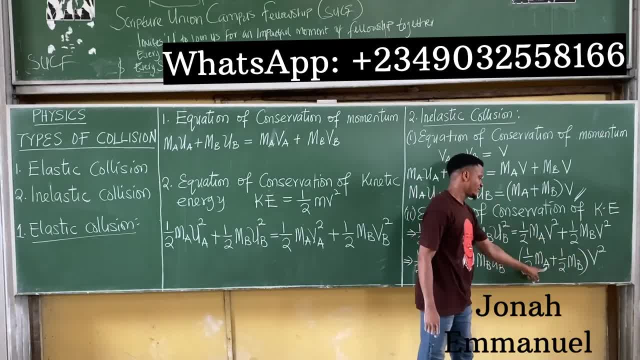 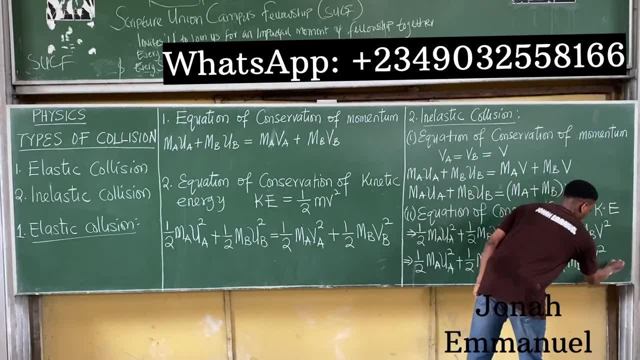 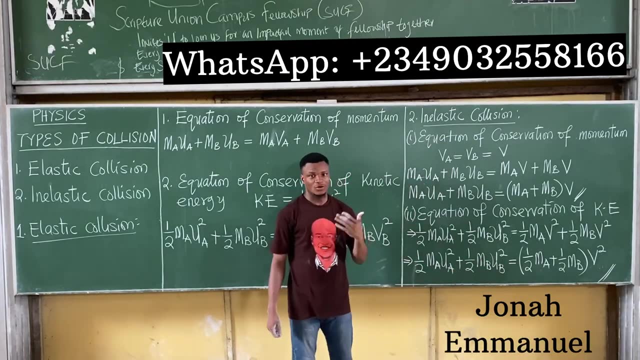 So you can confirm this: V squared times half m a gives you half m a v squared. Plus v squared times half m b gives you half m b v squared. So this becomes the equation of conservation of kinetic energy for an inelastic collision. 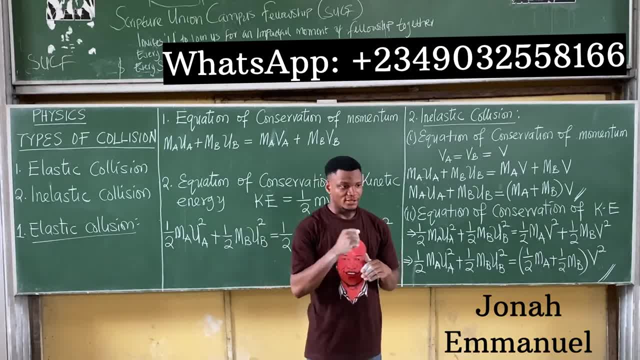 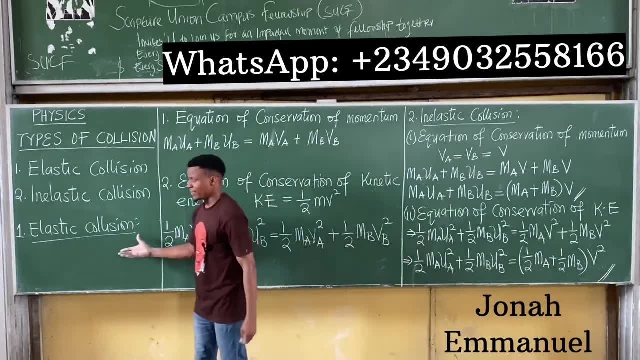 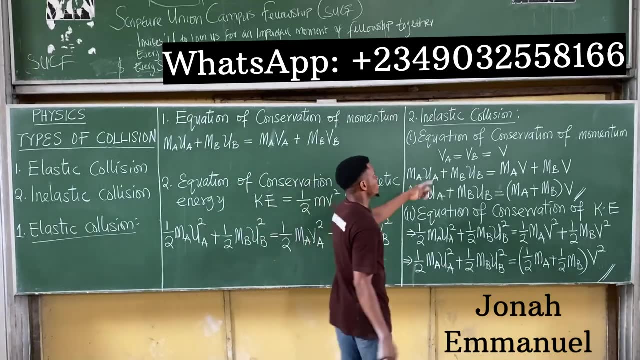 Alright, So that's it. So some differences between elastic collision and inelastic collision. The first difference is that for elastic collision the bodies collide and move with different velocities after collision. Why for? Because for inelastic collision the bodies collide and after collision they move with the same velocity after collision. That's one difference. 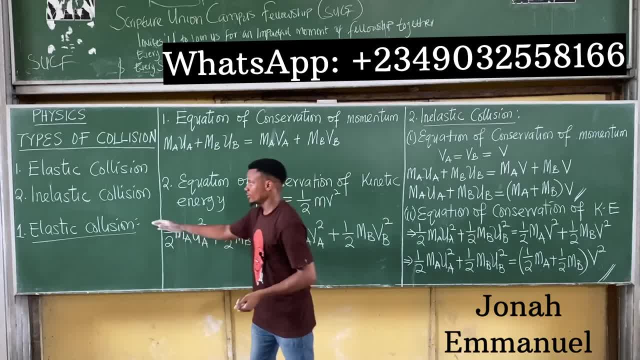 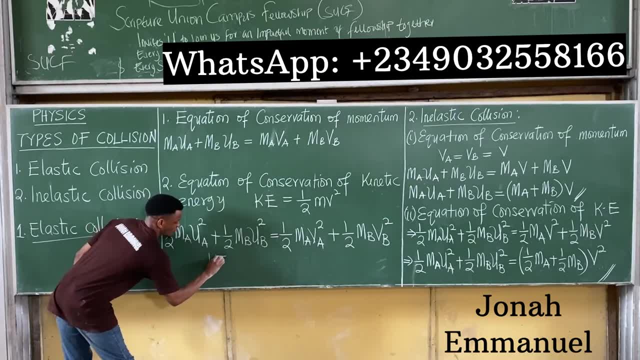 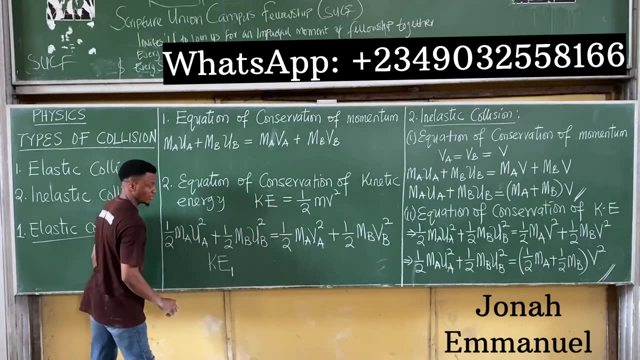 Another difference is that for elastic collision, as you can see here, the kinetic energy- notice this please: For elastic collision, the kinetic energy before collision is usual. Let's call this one. Yeah, Let's call this one. So one is before collision- is equal to the kinetic energy. 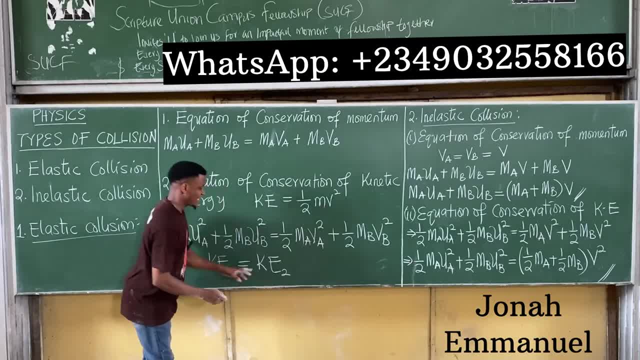 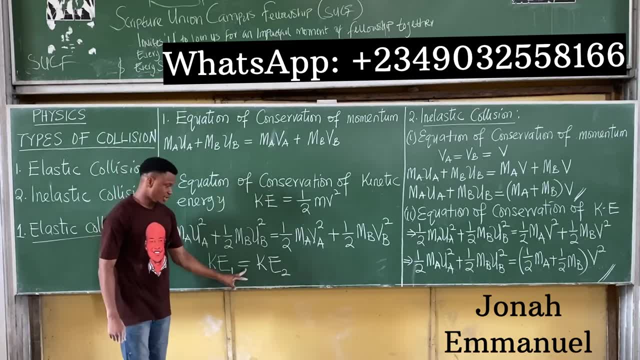 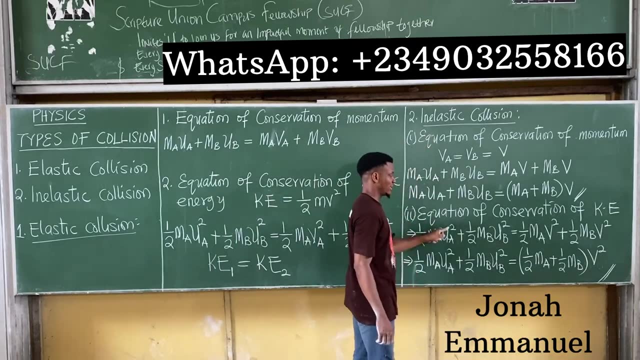 Let's call this two after collision. Please observe technically that for elastic collision the kinetic energy before collision is equal to the kinetic energy after collision. But when it comes to inelastic collision there notice that the kinetic energy before collision is not equal to the kinetic energy after collision. 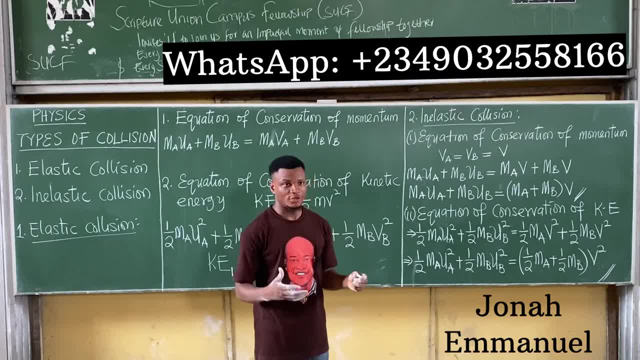 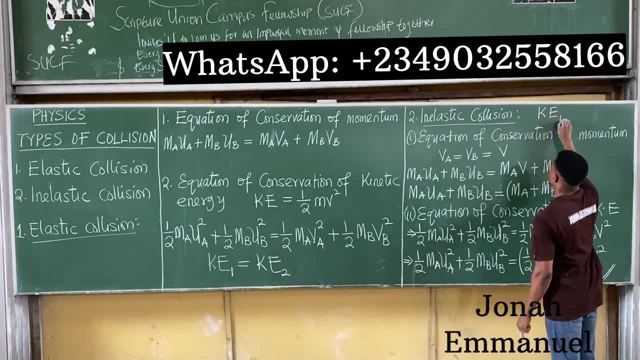 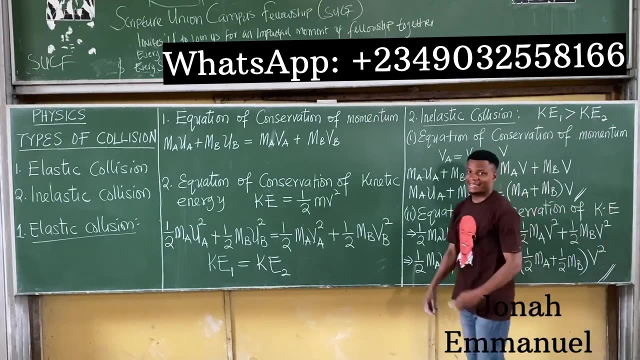 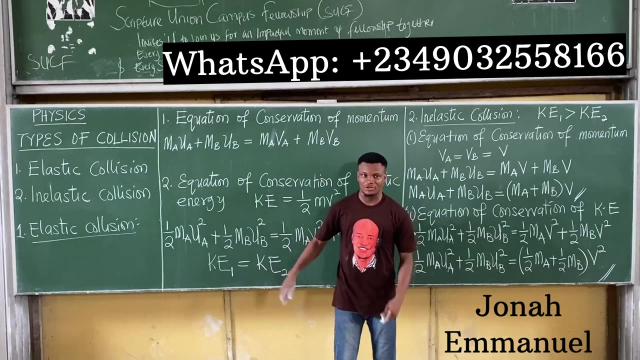 Alright. So energy is being lost after collision. So for this we can say that for inelastic collision, notice that the kinetic energy before collision is always greater than the kinetic energy after collision. So this is like a second difference. Alright, For this one. here the kinetic energy before collision is the same as the one after collision. 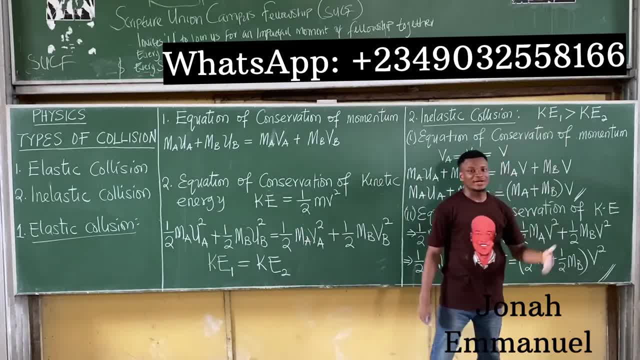 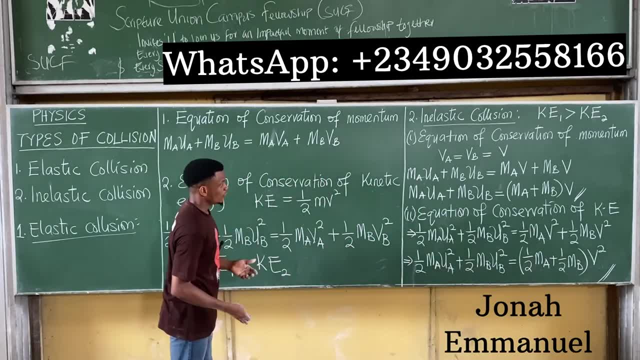 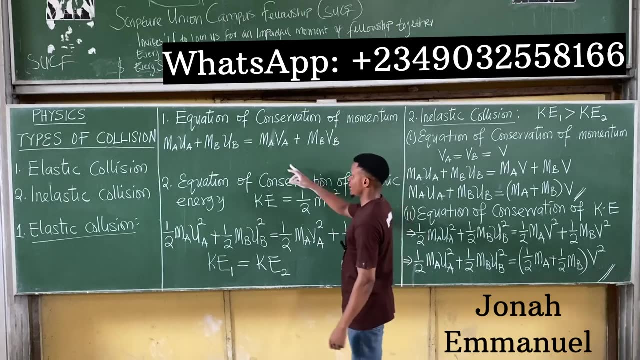 While for inelastic, kinetic energy before collision is usually greater than kinetic energy after collision, The similarity there would just be that for both of them we can say okay. also, note that for conservation of momentum. note that for conservation of momentum here. alright, you can see what the equation looks like. 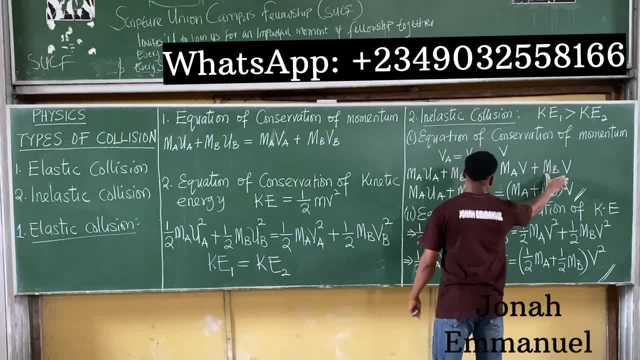 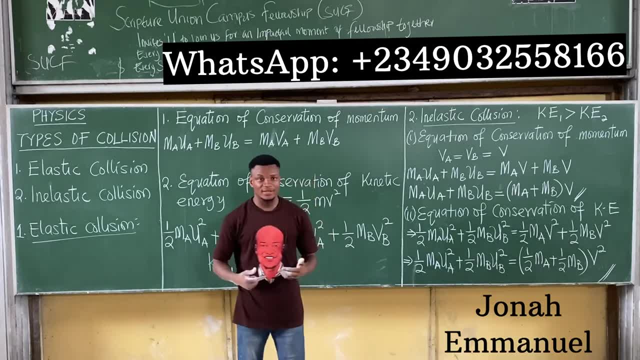 Okay, You have different velocities, You have here the same velocity, Alright. So this is like the difference between elastic collision and inelastic collision. We'll take some problems and then we'll solve for both of them, Alright. So this is like the difference between elastic collision and inelastic collision. 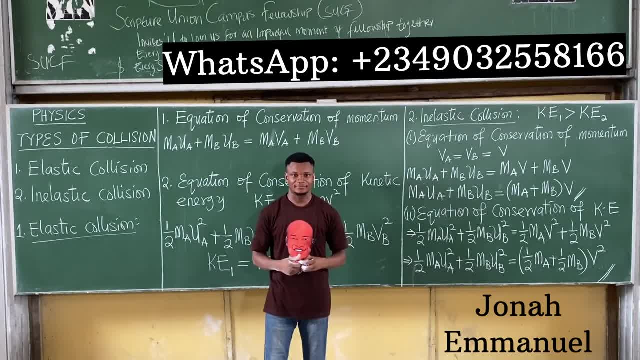 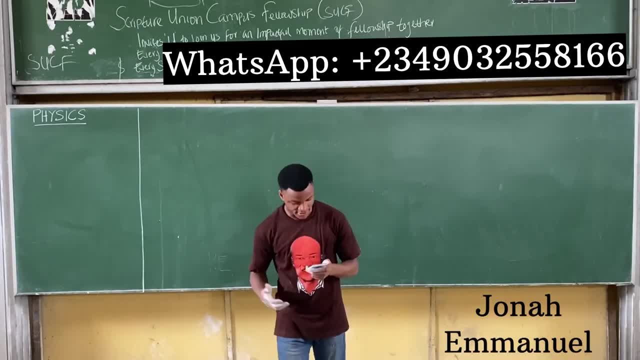 We'll take some problems and then we'll solve for both of them So you can understand them better. Alright, So let's take a sample problem on collision and see what we have. Alright, So let's take a sample problem on collision and see what we have. 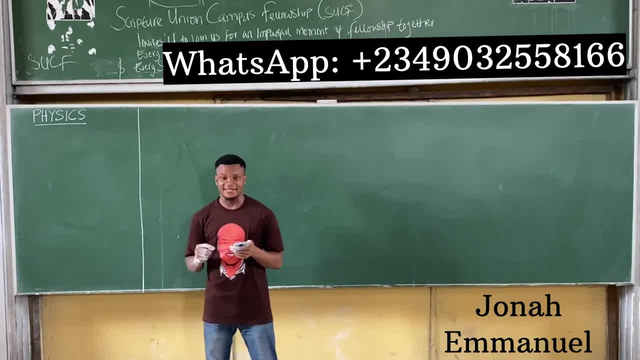 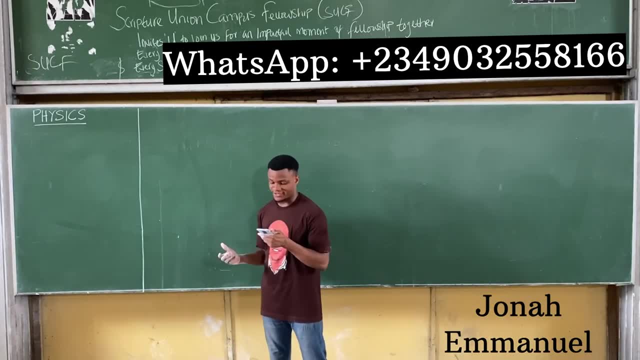 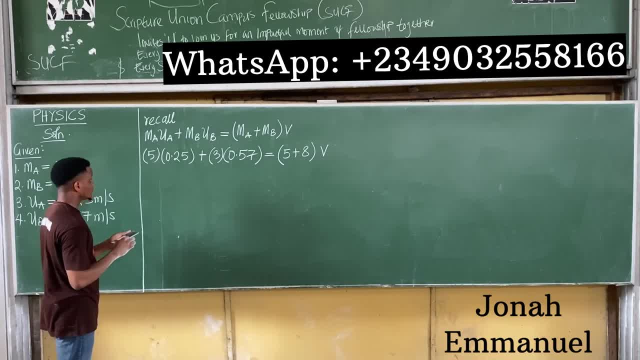 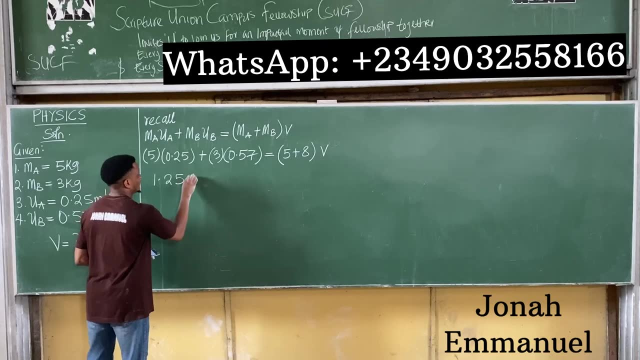 Now this equation says two bodies, A and B, of masses 5 kilogram, moves towards each other with velocities 0.25 meter per second respectively. Add to it the process of multiplying. Let's see What do I have there. To multiply it too, I have 5 times 0.25. 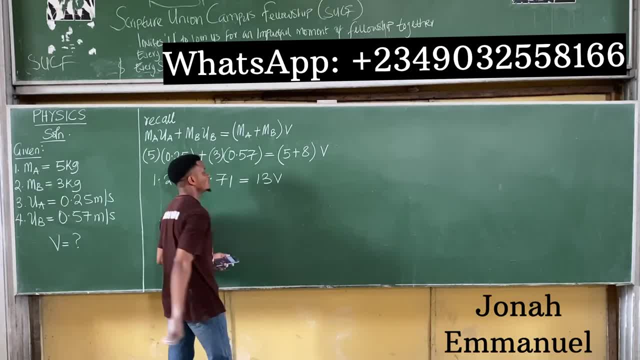 That's about 1.25 plus 3 times 0.57.. And that's about 1.71 is equal to 5 plus 8.. into V. That's why I have this. If I combine these two, I have. 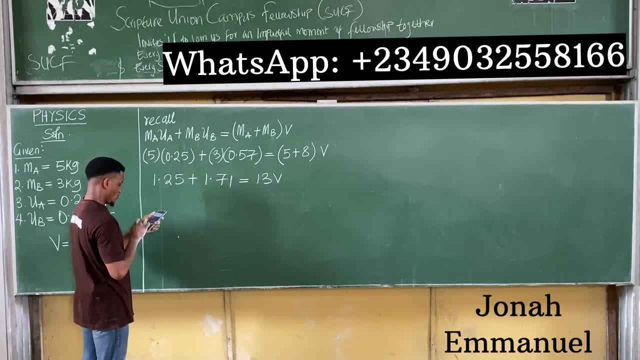 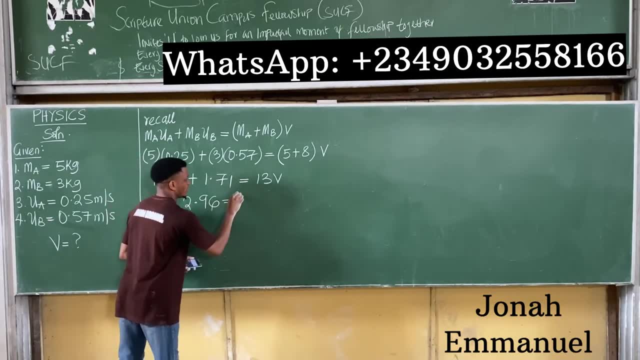 1.25 plus 1.71.. That's about 2.96 is equal to 13V. To get V, I'll divide it by 13.. Divide it by 13.. This cancels this. So it means that V is equal to. 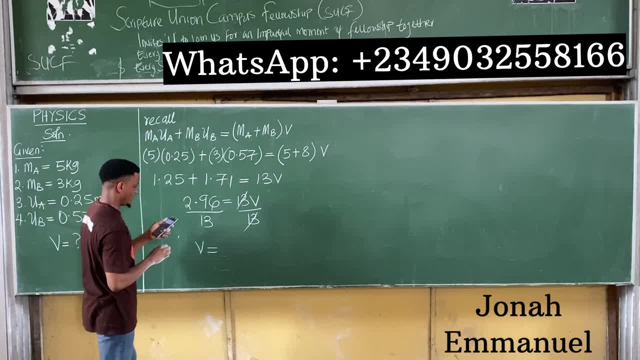 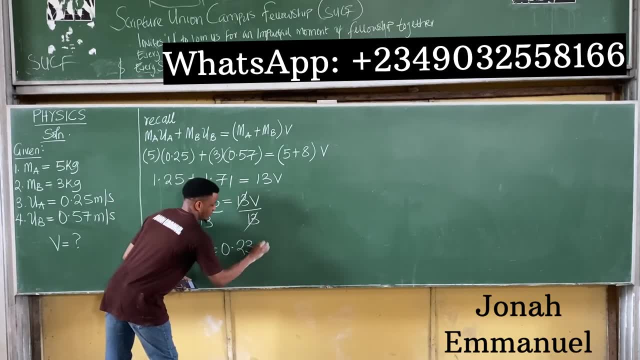 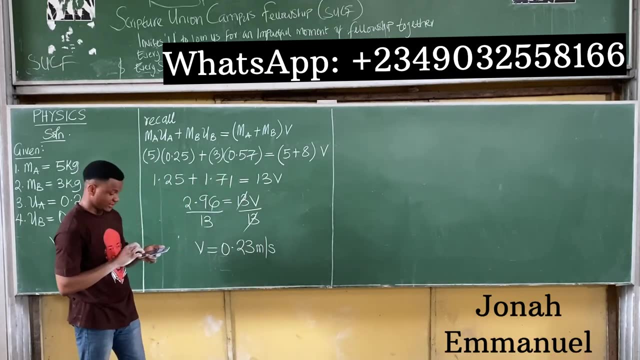 2.96 over 13.. I have 0.23.. Since this man here is velocity, it will be in meter per second. Hence this becomes the velocity of the bodies after collision. I've gotten the first one there as 0.23.. 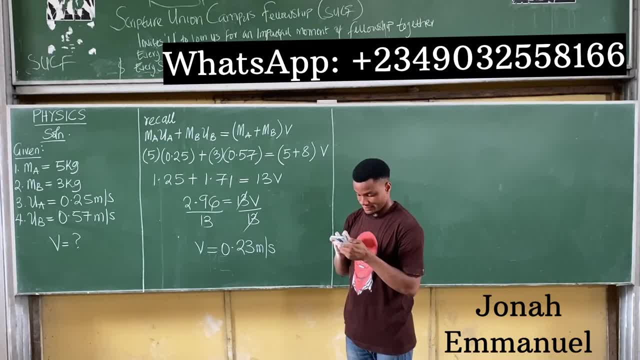 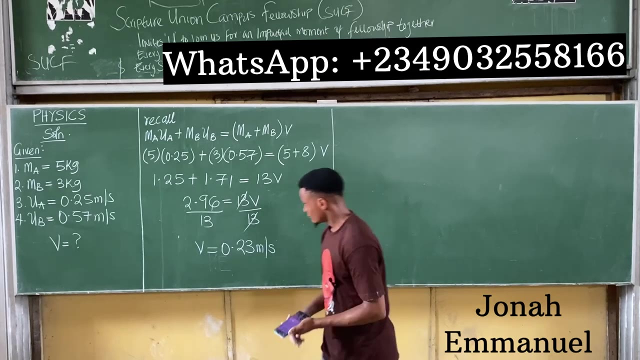 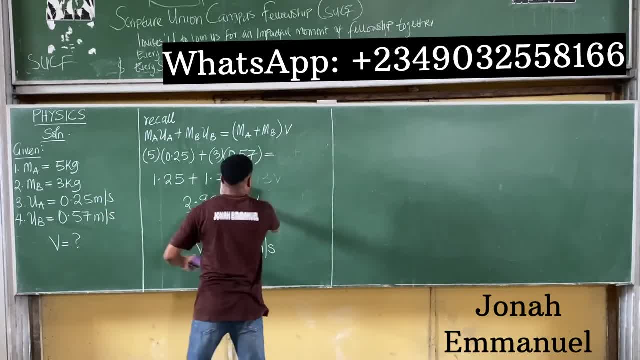 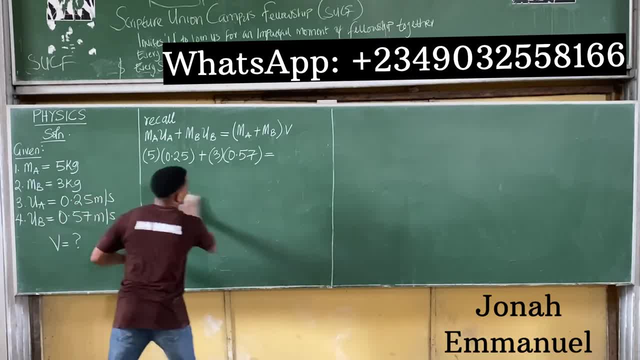 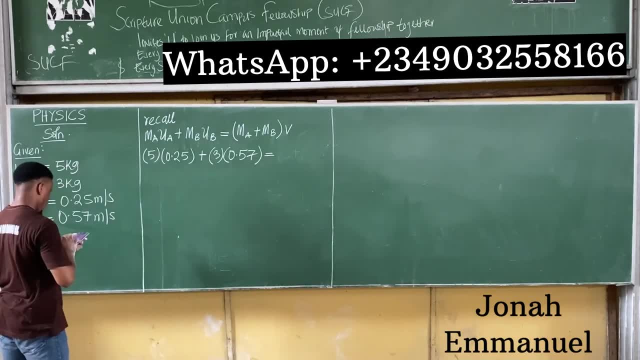 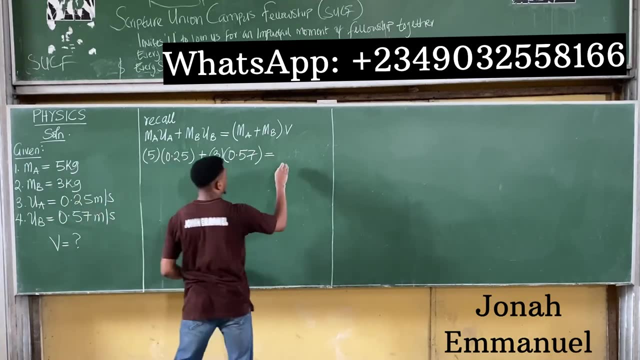 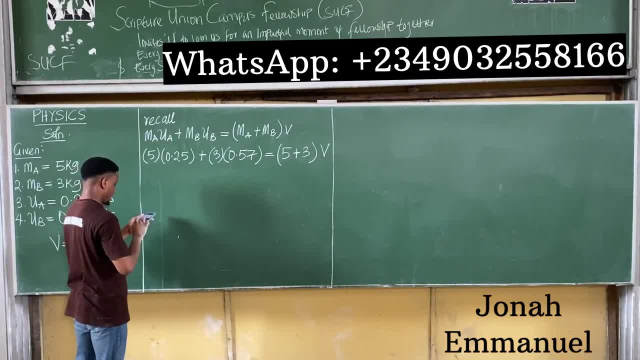 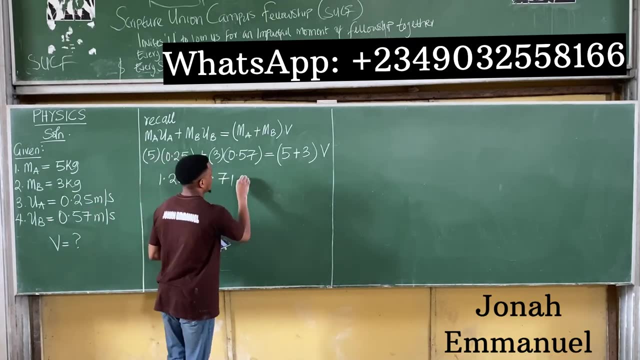 All right. so combining this, so 5 times 0.2, I have 3, and I have 3.. 0.25, I have 1.25, plus 3 times 0.57, I have 1.71, is equal to 5 plus 3,, that's 8 into v. 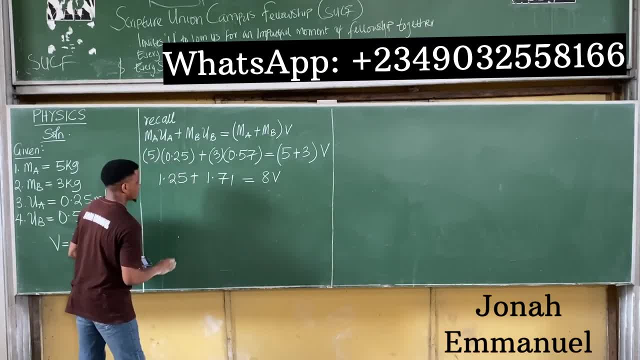 so 8v. if I combine these two, this gives me 2.96 is equal to 8v. to get the value of v, I will divide here by 8,, divide here by 8, so v is equal to 2.96 over 8, that's about. 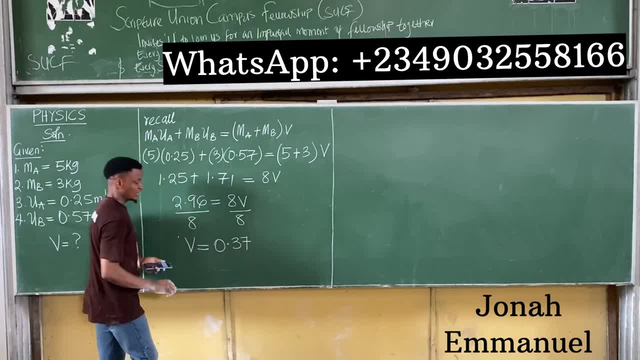 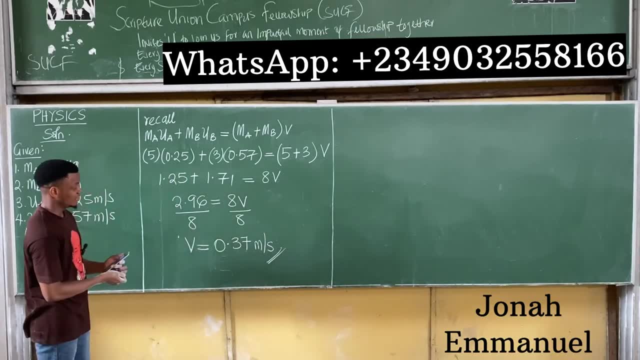 0.37,. now, since we are calculating for velocity, the unit will now be equal to 0.37, so we can be meter per second. so I have 0.37 meter per second as my result. alright, so I've gotten. 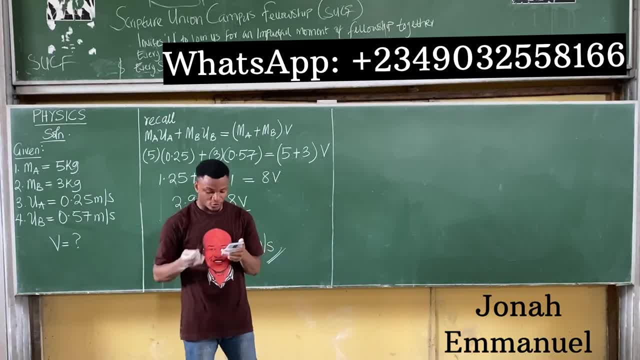 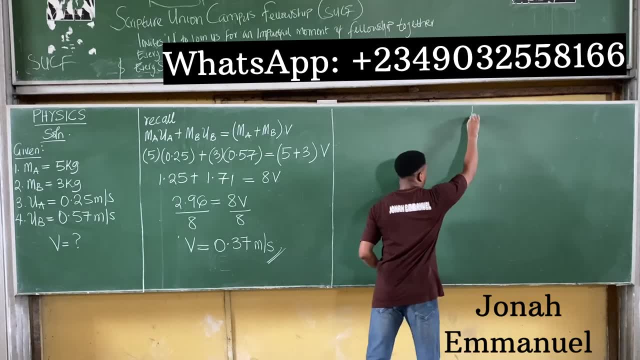 the first one there. the next one we are asked to do is to find the total kinetic energy of the system before and after collision. alright, let's get kinetic energy before collision, kinetic energy after collision. alright, let's call it b part kinetic energy. 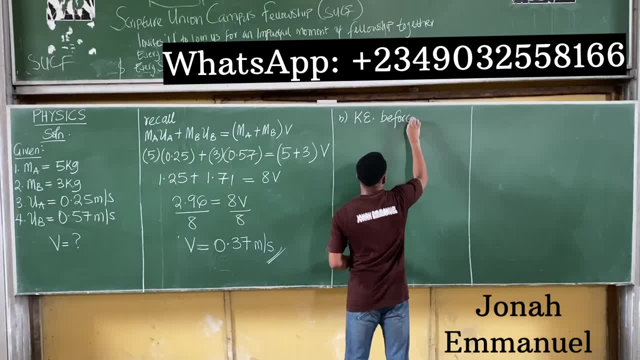 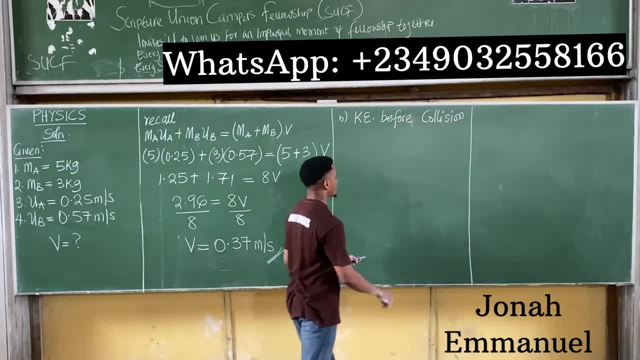 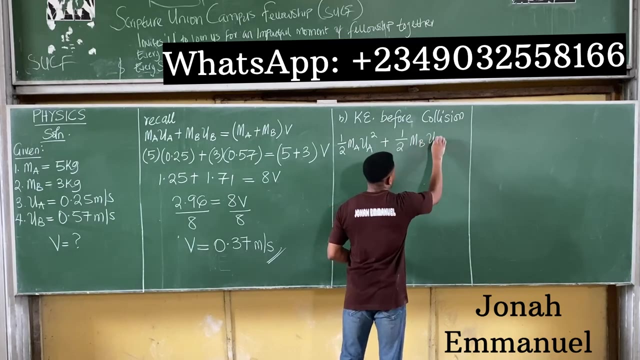 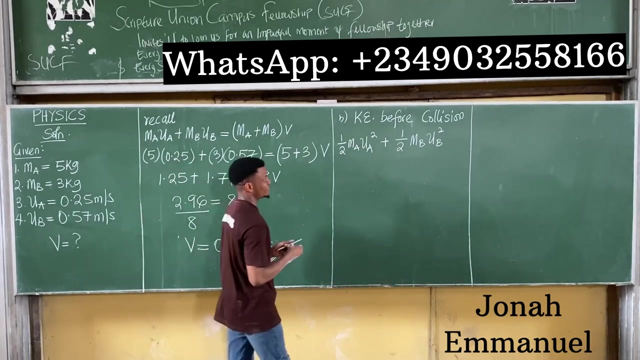 before collision. now recall my formula, that we had the formula for this as half m a- u a squared plus half m b- u- b squared. so that's just simply the left hand part of that equation, which was this: that's how we get the kinetic energy before collision, if I impute values. 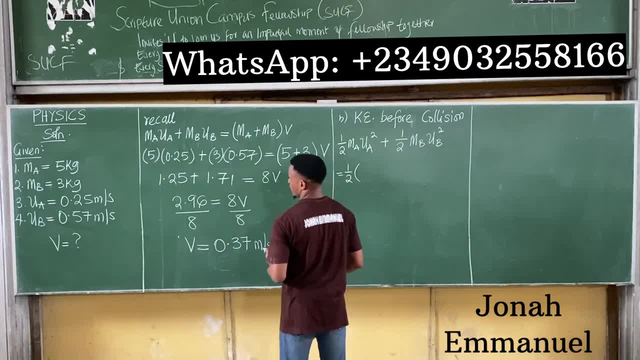 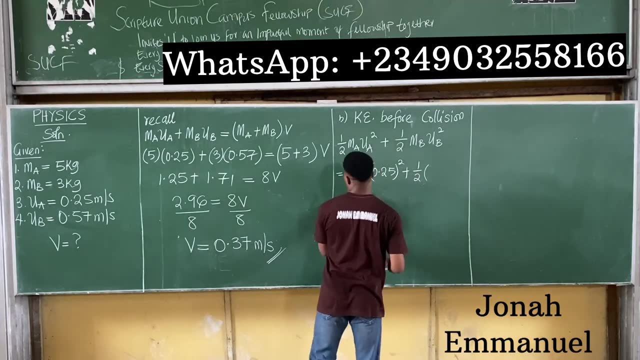 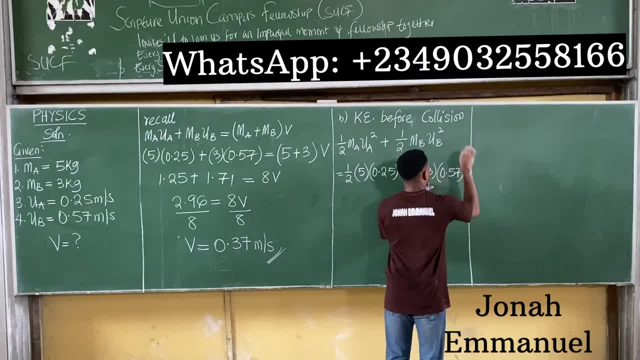 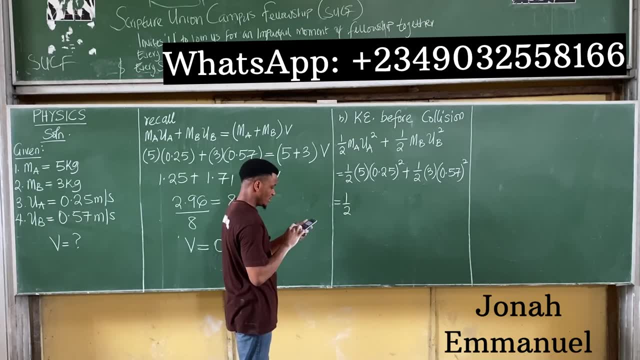 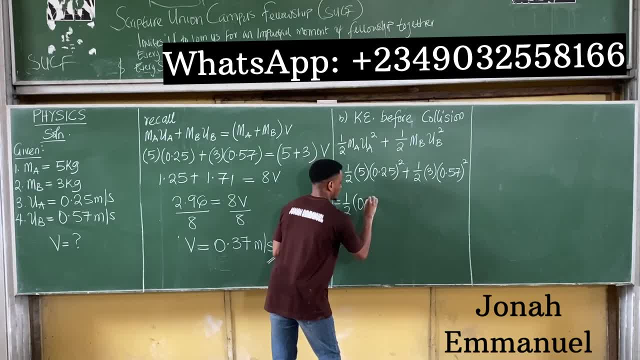 this. that gives me 0.3125,. so please make sure you're punching your calculator correctly, or if you're not sure, you can just punch 0.25.. 0.25 squared First when you get your answer. you now do times 5, you would have this one here, okay. 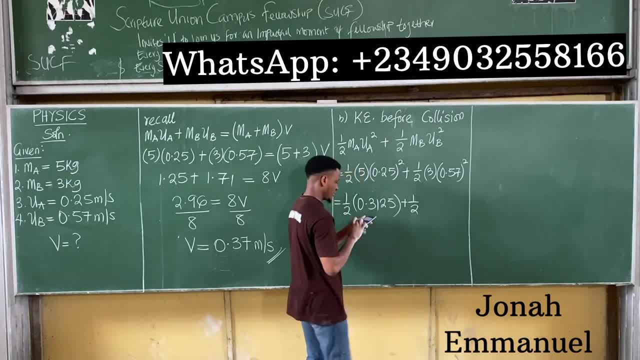 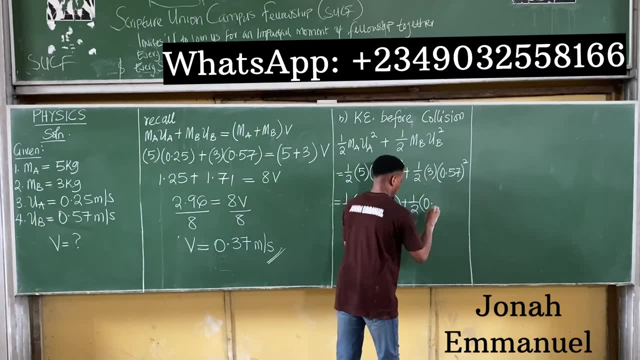 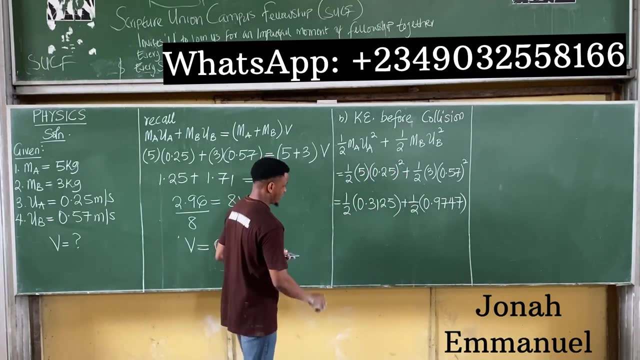 plus half into 3 times 0.57 squared, and that's about 0.9747, 0.9747,. alright, so take half of this and see what we have: 0.9747.. 0.9747.. 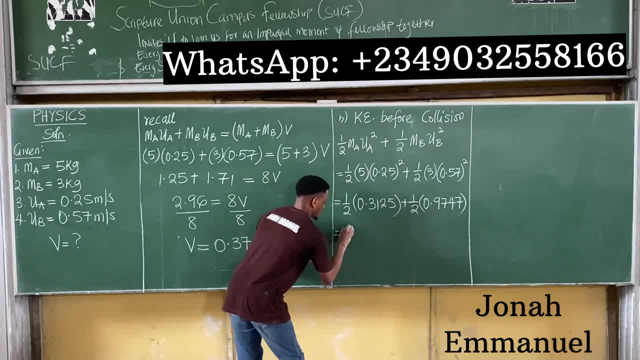 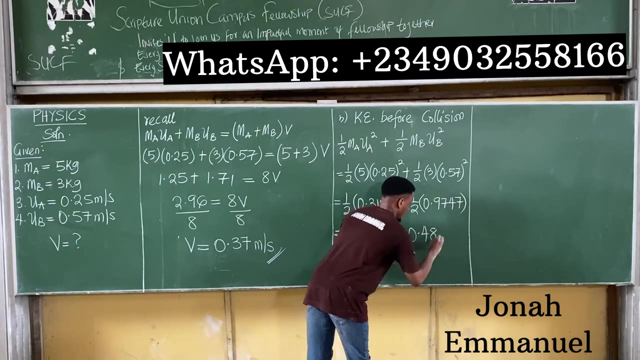 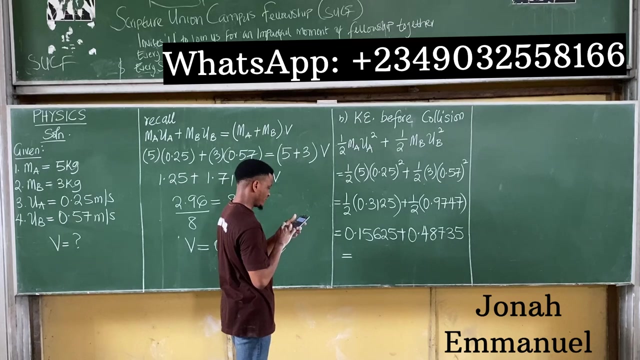 So we take this 0.3125 and that's about 0.15625, plus get this one here half times 0.9747, that's about 0.48735.. If I combine these two that would be equal to 0.15625 plus 0.48735.. 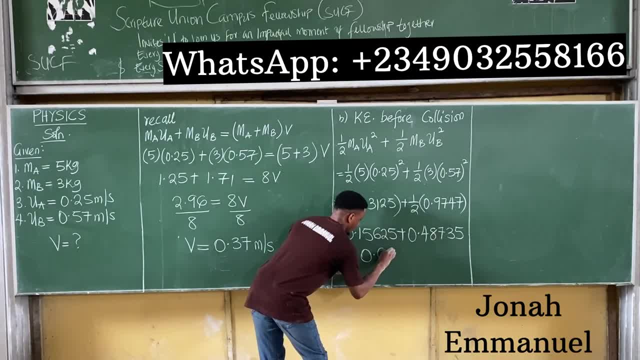 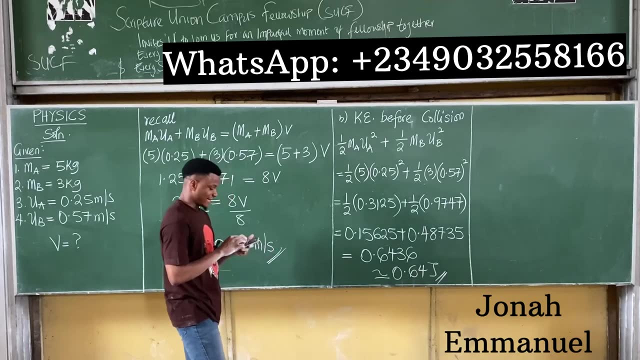 That's about 0.6436.. In two decimal places, that's 0.64.. Kinetic energy is measured in joules, So I have 0.64 joules as the kinetic energy before collision. Let's get kinetic energy after collision. 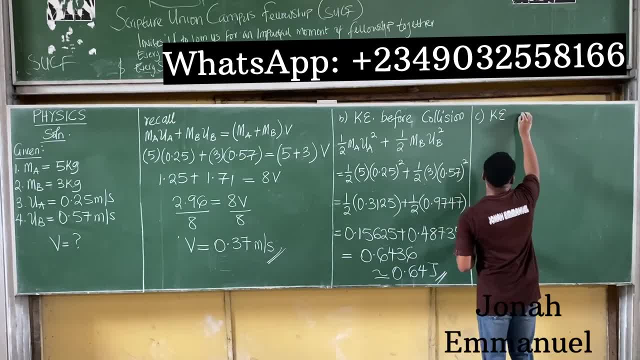 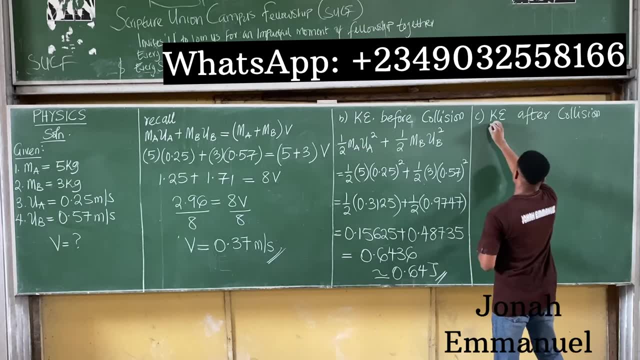 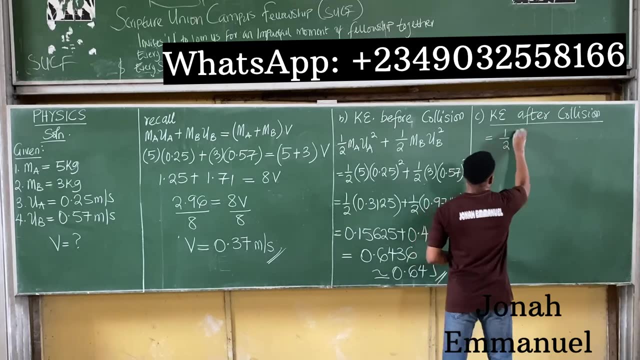 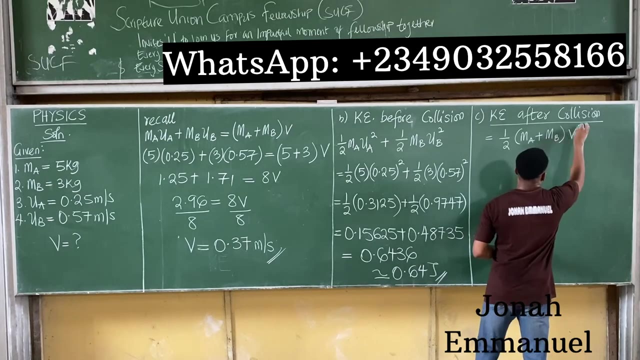 See kinetic energy after collision. Now check the equation again. Check the right-hand part of the equation. We said we would have something that looks like to be equal to half into MA plus MB, into V squared, Something of this nature: 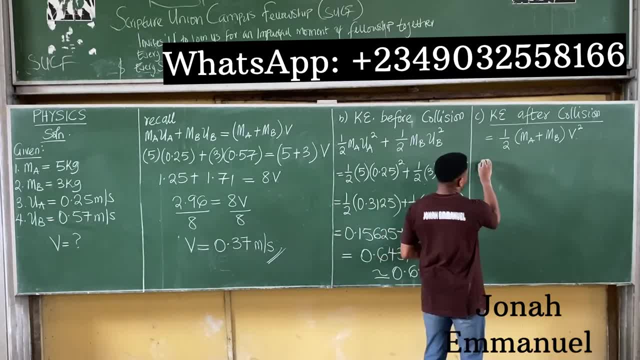 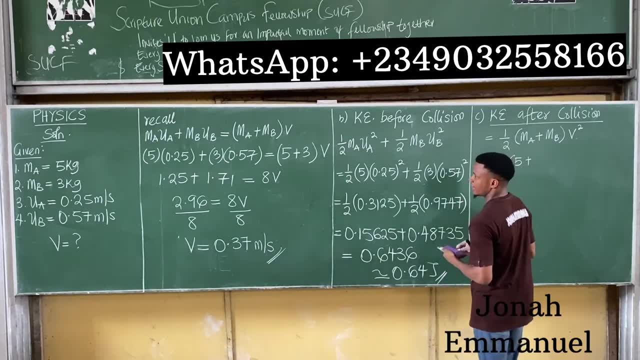 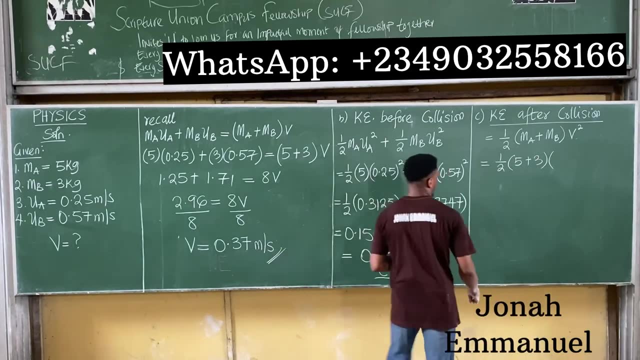 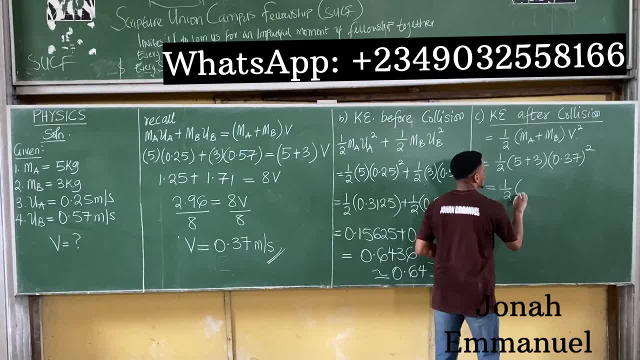 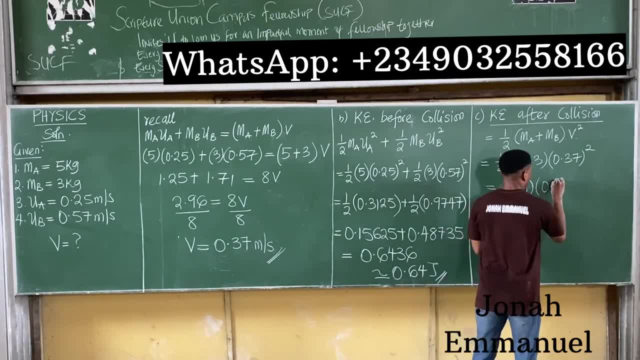 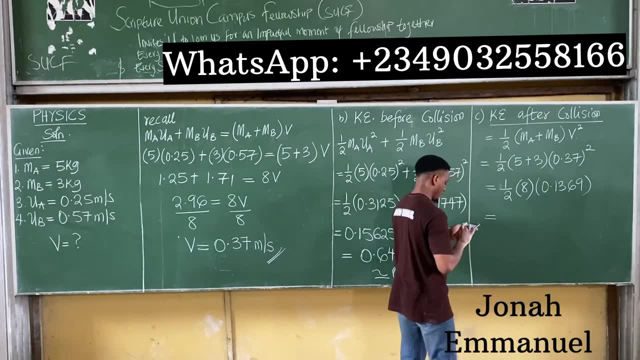 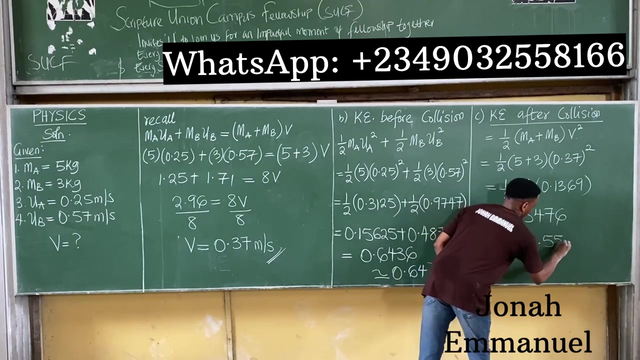 That is about 0.1369.. Alright, so multiplying through that's equal to half. So half times 8 times 0.1369.. 0.1369.. 0.1369.. about 0.5476.. Approximately, in two decimal places this would be 0.55 joules. So I have. 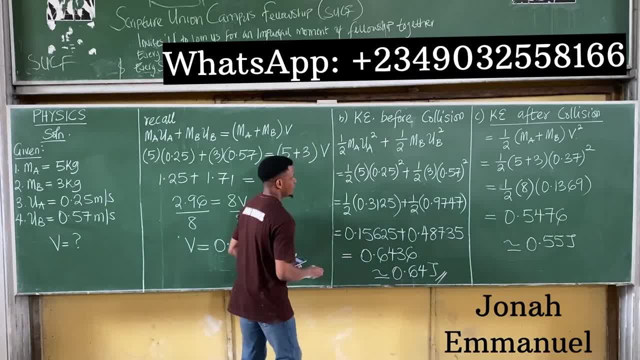 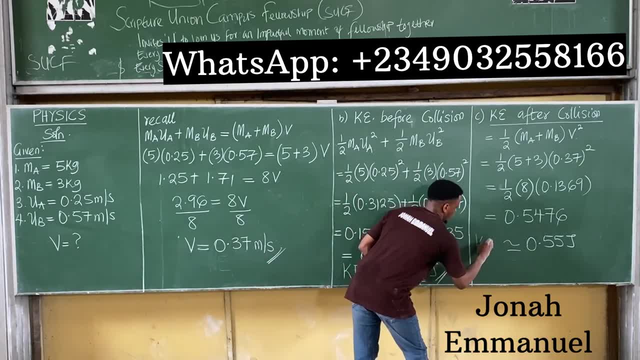 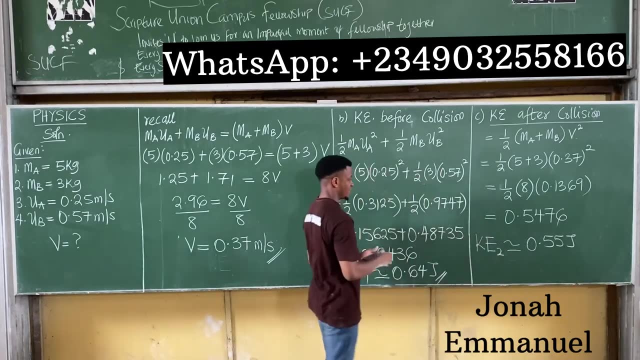 this. All right. So this is the value of the kinetic energy: before collision. Let's call this Ke1.. That's before collision. Let's call this. after collision. Let's call this Ke2.. All right, So we have this, Our last task here. last question here is to hence: 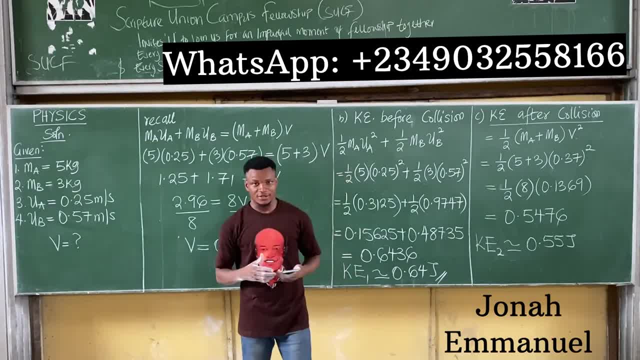 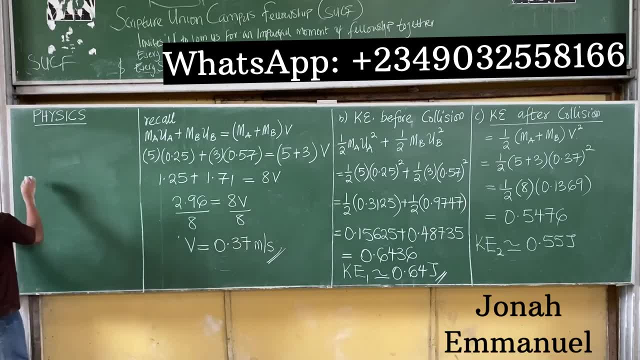 calculate the loss in kinetic energy, That's to find loss in kinetic energy, All right. So the last part there, let's call this D: The loss in kinetic energy would be equal to the difference between the initial kinetic energy and the final kinetic energy. This 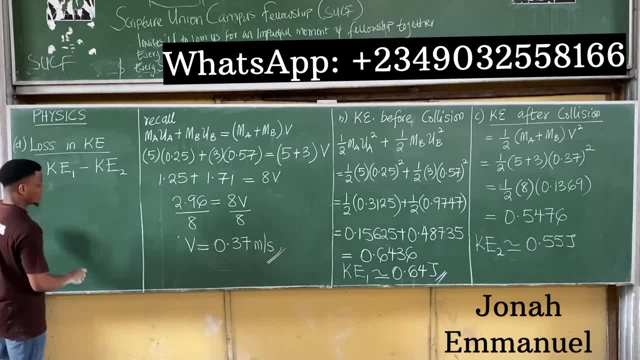 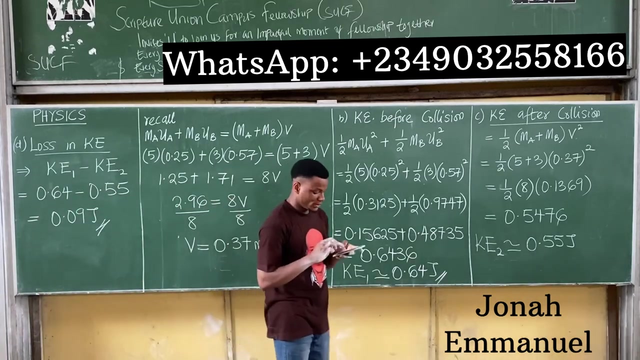 is equal to the initial kinetic energy is 0.64, 0.64 minus the final kinetic energy is 0.55.. So how many has been lost? We have 0.64.. Minus 0.55. That's about 0.09 joules approximately. So 0.09 joules is the value for the loss in. 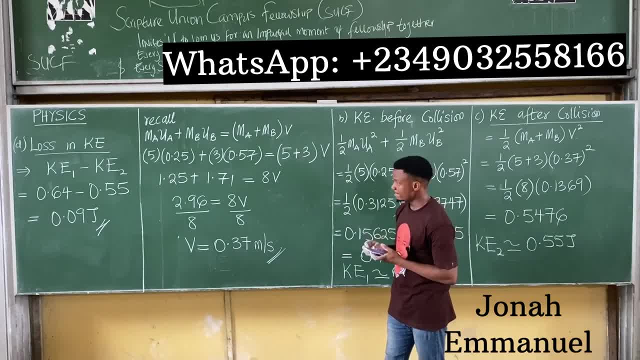 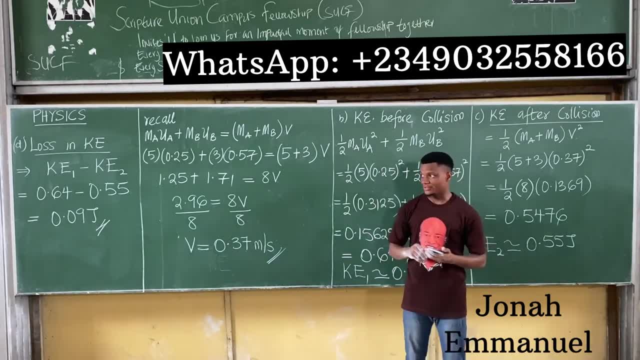 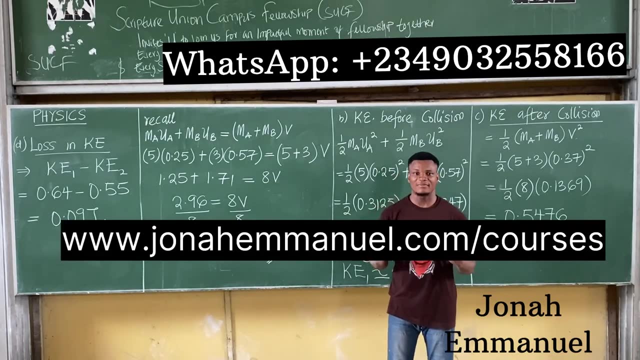 kinetic energy of this system. All right, 0.09 joules. All right. So this is how we solve this question. All right, So I've prepared over 50 plus classes. All right, So let's move on. So I've prepared over 50 plus classes on physics, chemistry, mathematics and other.